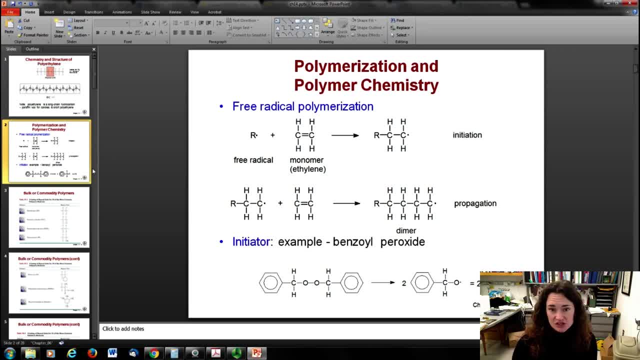 of ethylene. You want to make polyethylene. So let's say that you take your ethylene and you have this double bond here. Well, you introduce something that's got this dangling electron, this free radical, and it reacts, breaking that double bond. Now, of course, 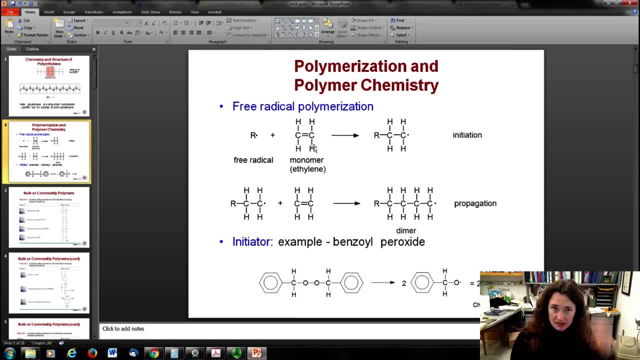 remember we discussed that double and triple bonds are easier to break than they're less stable than other sorts of bonds. There are a lot of monomer units and so that bond breaks relatively easy. When it sees this electron over here, it's just too tempted and it breaks that double bond and then it. 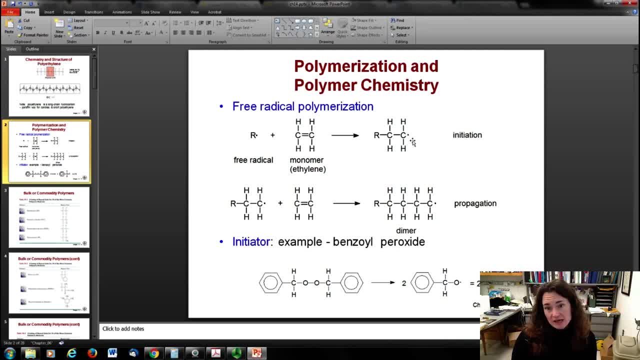 hooks on there. Of course, when it breaks the double bond, then the carbon on the right-hand side it has a free electron because the double bond's been broken and it has four available bonds. And so what happens is it then becomes the free radical and continues on propagating. 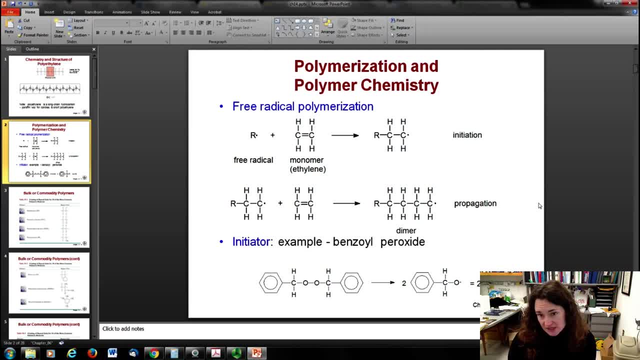 the reaction through. So it propagates until you stop it And by introducing some other sort of chemical to cut it off, you can initiate the reaction with something like benzoyl peroxide to form the free radical. Like I said, there's whole. 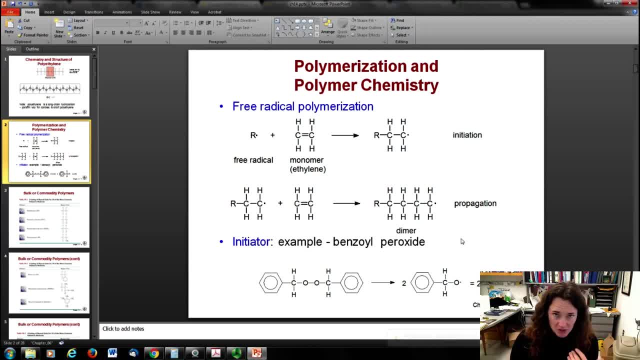 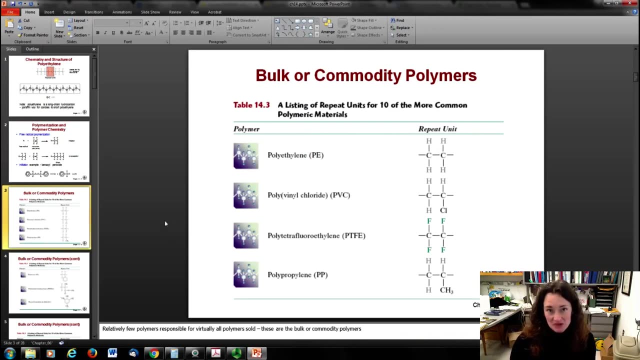 areas of chemistry that are totally devoted to this. People get PhDs in polymer chemistry, But that gives you kind of a general idea of how polymers are created from monomer units, And there's way more than one way. OK, So that's just one way. Many, many reactions. 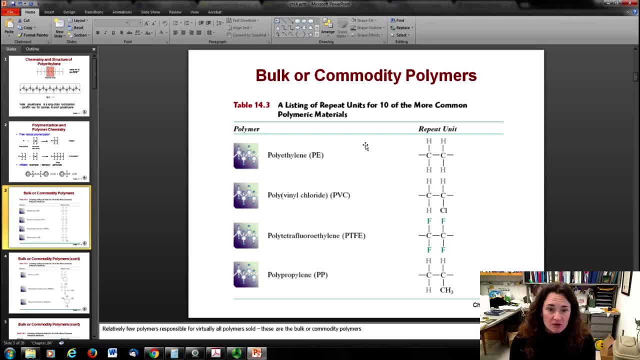 can trigger it OK. So, in terms of some of the polymers that are out there, you're probably familiar with a lot of them just from looking at the recycling symbols on the bottom of the things that you use. So we've got polyethylene here. It's often abbreviated PE. You might see on the. 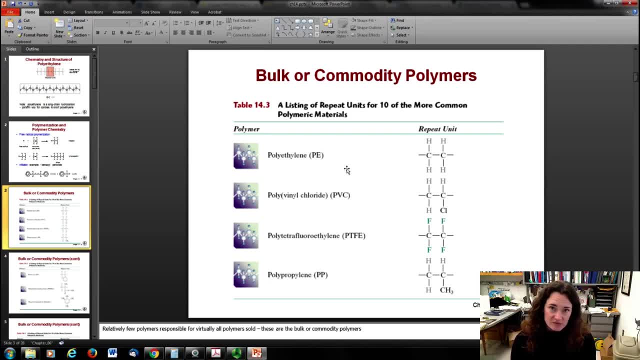 bottom of your recycling: HDPE or LDPE, That stands for high-density polyethylene or low-density polyethylene. So those are very common recycled materials. Polyvinyl chloride or PVC. that's two carbons, It's with a chlorine on one side and then three hydrogens put together in a long unit. 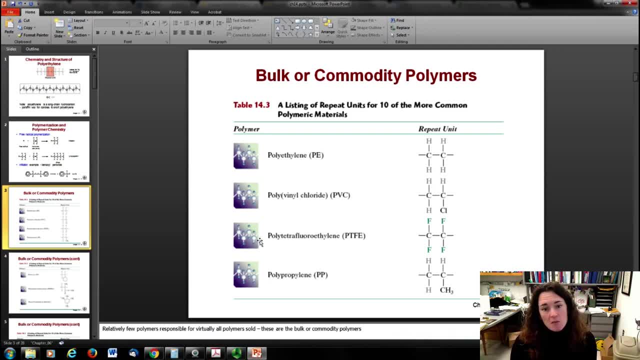 PVC pipe. you're probably familiar with PVC- Polytetrafluoroethylene. the trade name for that is Teflon, But it's abbreviated PTFE, So you're probably familiar with Teflon coatings on your pants- the nonstick coating. 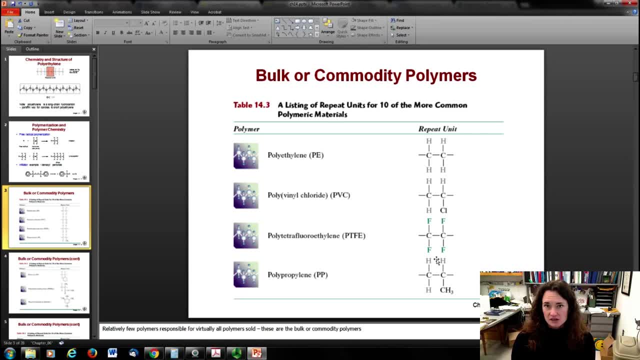 Of course that's because the carbons here are bonded to fluorines on all sides, And the fluorines are very, very happy to be bonded, And so they're very nonreactive. They don't even want to react with sodium. 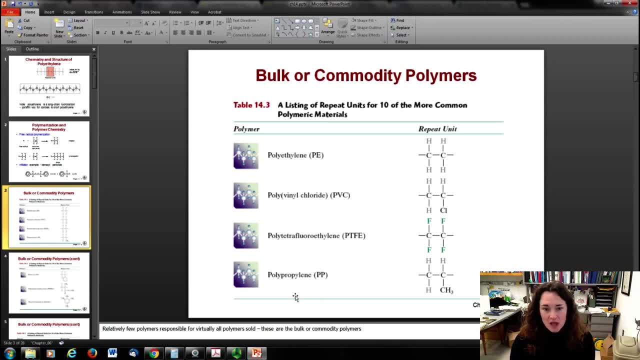 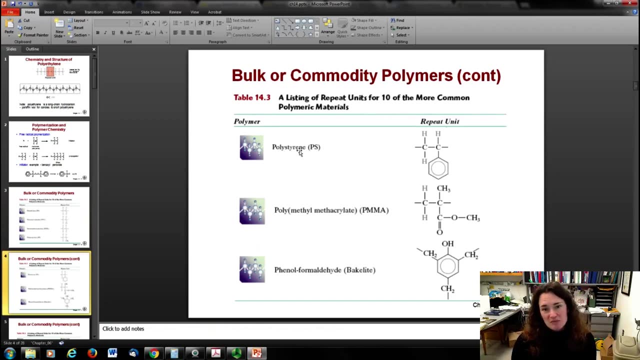 Polypropylene. you've probably also heard of PP. it's on a lot of plastics that you get the recycling symbol on the bottom. A lot of plastic containers are polypropylene- Polystyrene- these are the little styrofoam peanuts that you might see in packing materials. 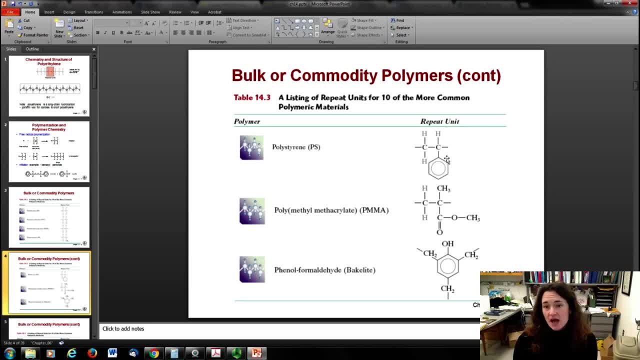 It's also styrofoam, which makes up a lot of seat cushions. In that case you have these carbon atoms in the chain bonded to the fetal group down here on one side: Polymethylmethacrylate or PMMA. This is a really common photoresist When it's exposed. 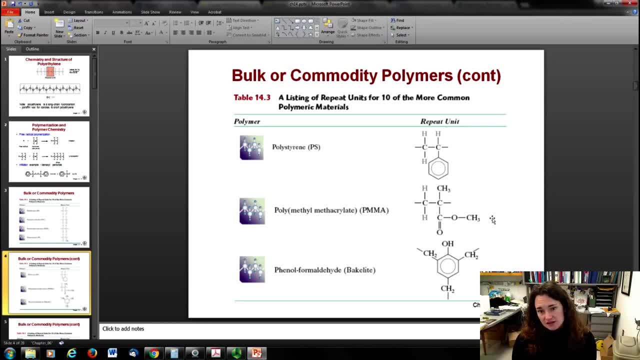 to light. it's very reactive And so it gets used a lot in semiconductor manufacturing and things like that- Phenol, formaldehyde or bakelite. It's a really old school plastic. Some of the very first plastic dishes that went on the market were made of bakelite, But it doesn't respond very. 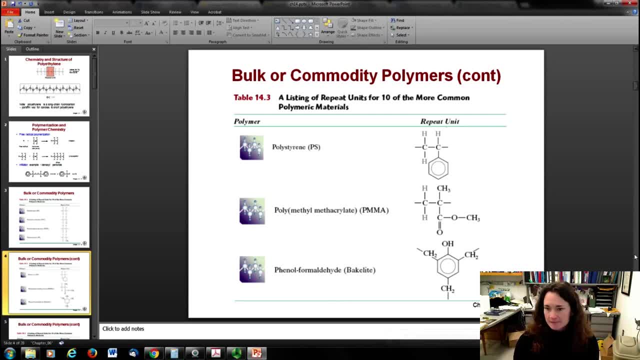 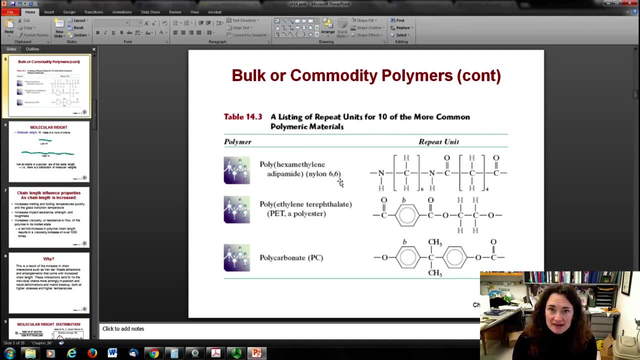 well to heating, so it's not very popular today. Continuing on Nylon 66. We're going to do a lab in making nylon in the laboratory, But Nylon 66 is also, of course, nylon fibers present in a lot of clothing: Polyethylene. 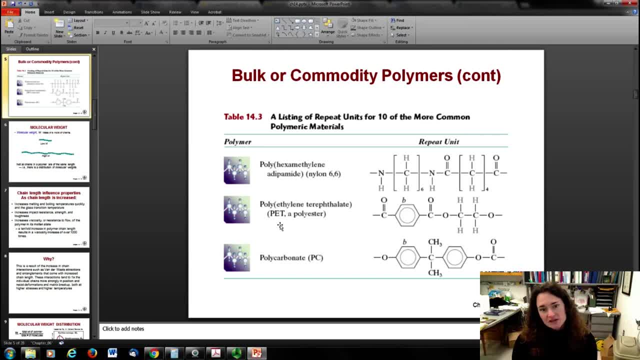 terephthalate makes up all the soda pop bottles. So the PET bottles, Coke bottles, soda pop- all made of that. Also, polyester fabrics are made for that, So your fleeces, things like that, are made out of polyester, And then the other things that are made of polyester. 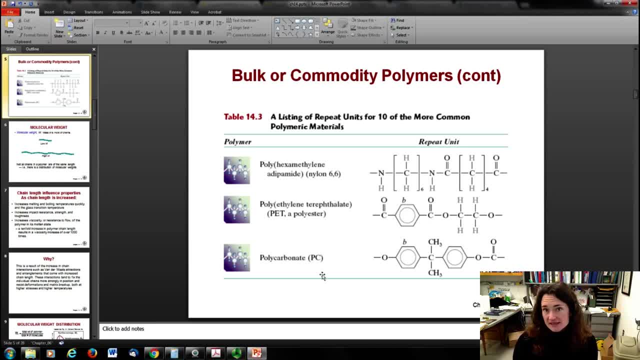 polychloricverts, Poly��as, And polycarbonate is a very glossy polymer, So spit guards on salad bars and things like that of polycarbonate, And it also makes up the lenses of a lot of glasses out there- eyeglasses. 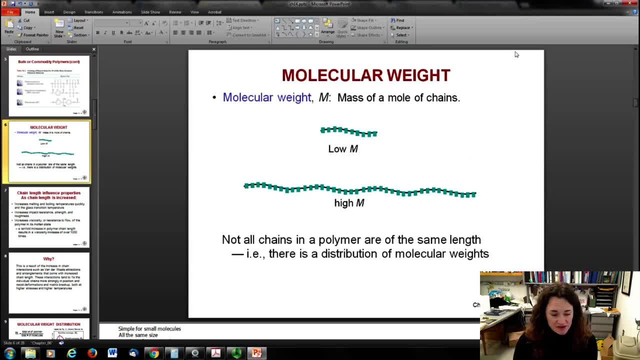 Molecular weight is one way to characterize and quantify some of the properties of a polymer. Basically, the molecular weight's a mass of one mole, of a whole, The molecular weight's of the polymer chains. okay, so high molecular weight polymers might have very different physical properties from low molecular weight polymers. and what 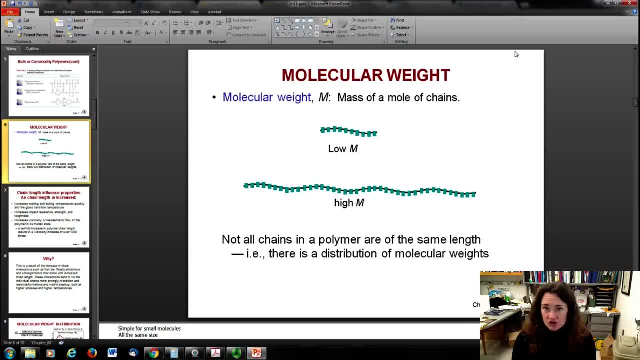 you want depends upon what application you're going to use it for. so not all chains in the polymer of the same length. so when you buy, say, a hundred thousand molecular weight polymer, you're going to get a distribution. there'll be a statistical distribution with the distribution kind of centered near the 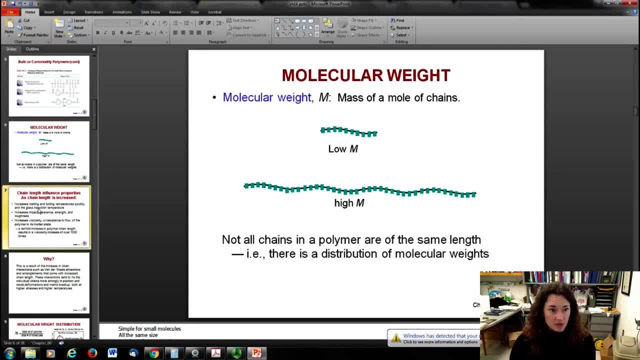 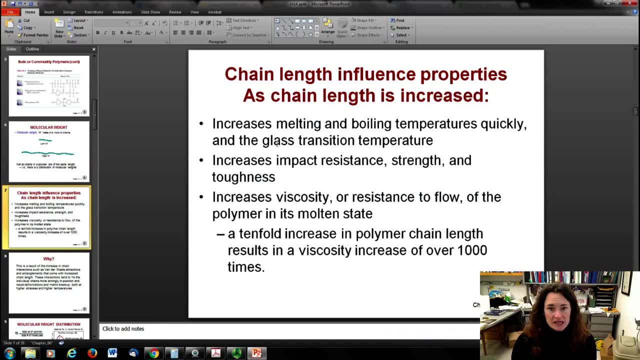 molecular weight side of on the bottle from where you bought it. now the molecular weight impacts the properties of the polymer in the following ways. as you increase the length of the chain, it increases the melting and boiling temperatures very quickly. it also increases what's called the glass. 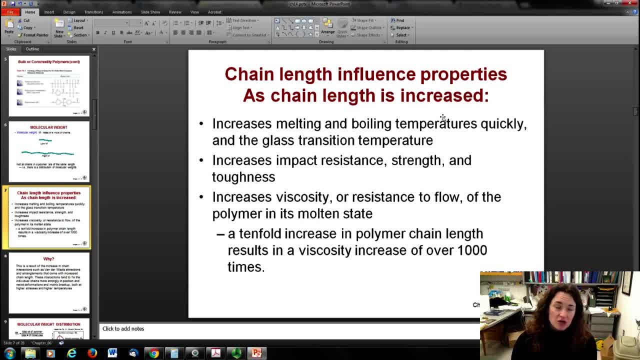 transition temperature, and that's the temperature at which a polymer goes from acting like a hard and glassy material to a rubbery and soft material. increasing the molecular weight also increases the resistance of the material to impact. it increases its strength and increases its toughness. it increases its viscosity. if you're not familiar with this term, the 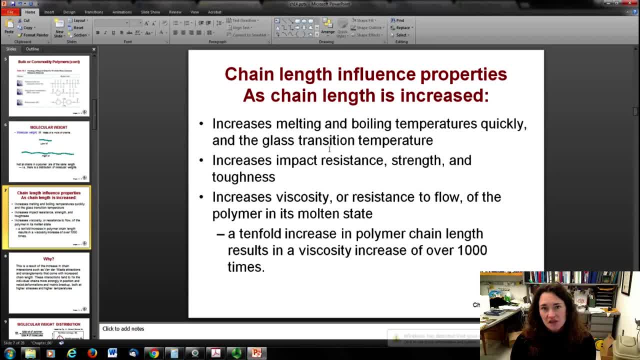 viscosity is a materials resistance to flow, so maple syrup, for example, is a lot more viscous than water. so a polymer's viscosity can be increased as the molecular weight is increased of the polymer when it's in its molten state. this can have very large impacts on the processing of parts manufacturing or 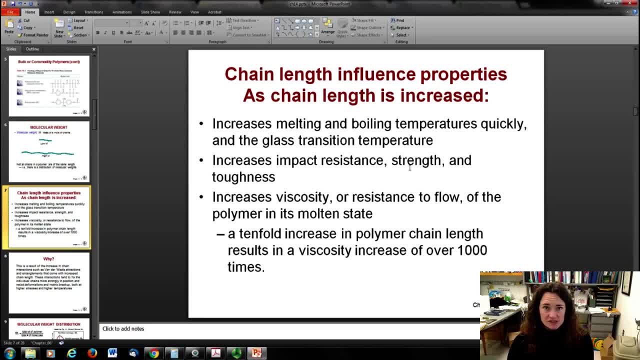 of parts for plastics for different applications. for example, if you want to mold, inject molten polymer into a dye and then allow it to harden, how easily that polymer flows into the mold is going to depend upon its molecular weight. to a certain extent you can get a tenfold increase if you increase the 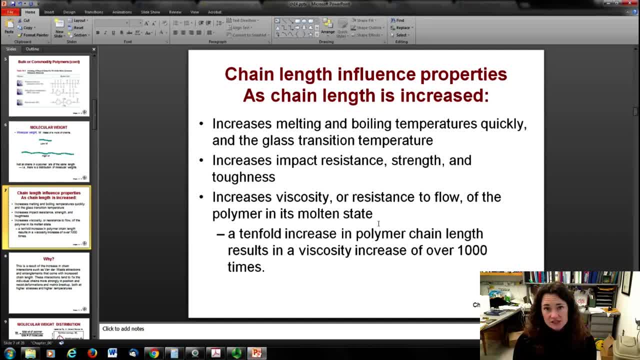 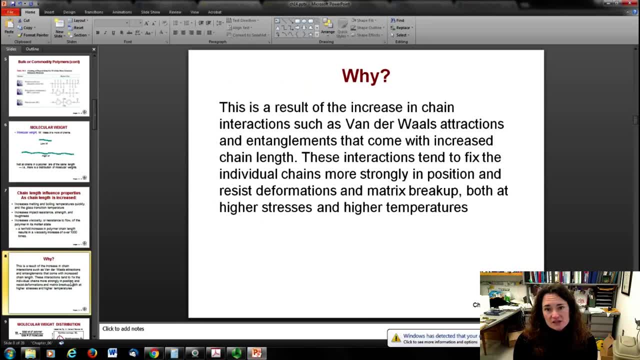 polymer chain length by tenfold and that results in a viscosity increase of over one thousand for the polymer. so you can see it has a huge impact. why? well, the reason is it's a result of the increase in the chain interaction. so, if you can imagine, a polymer is like a big, long piece of spaghetti and then it's laying. 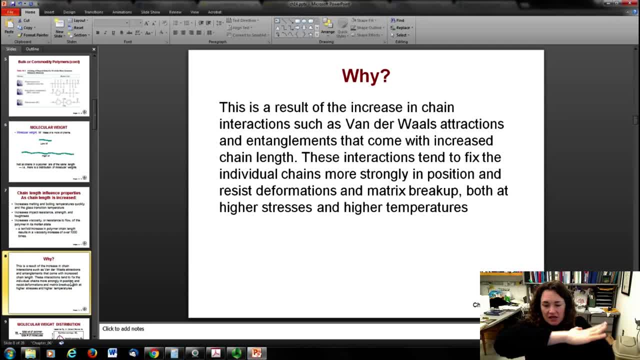 next to another piece of spaghetti. then the longer the chain is, the larger those weak bonds, or van der waals bonds, are between chains and the stronger it becomes. that means that it's going to entangle more with neighboring chains as the chain gets larger and the interaction tend to fix the individual. 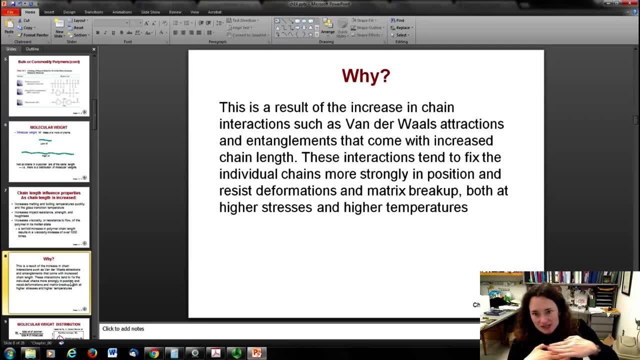 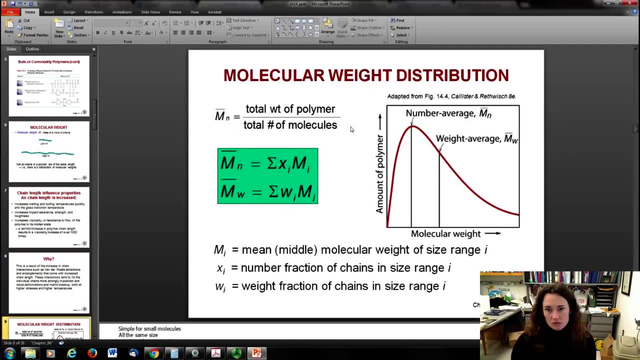 chains more strongly in position, and that means they're going to resist deformation and breakup of the matrix that's formed, both at higher stresses and temperatures. okay, one thing that you probably need to understand if you're ever going to be ordering uh polymers for any kind of application from a chemical supply. 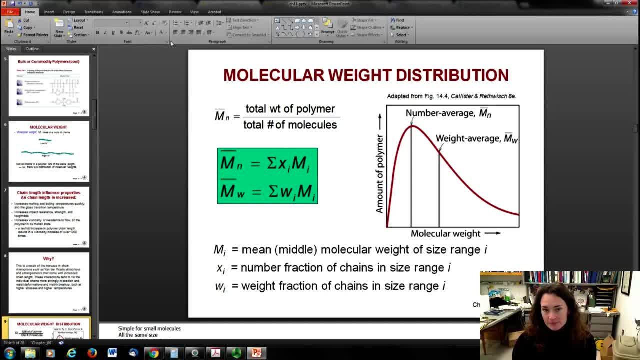 company is how these molecular weights are calculated. so there's two different kinds of molecular weights that get cited generally. when you polymerize, when you go through a polymerization process, you're going to get a distribution of molecular weights. now this isn't necessarily a symmetric distribution. it's got a tail. it looks like that. 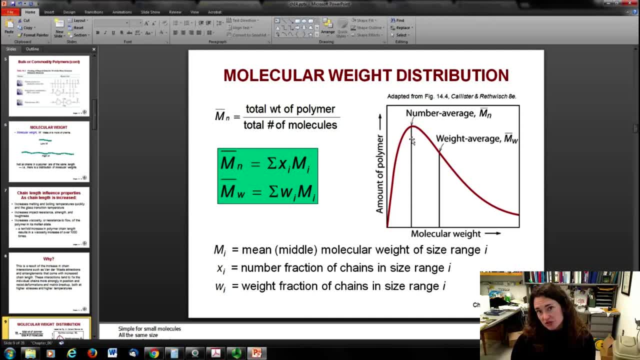 that means that since it's not symmetric, you can use a couple of different numbers to characterize that distribution. one is the number average molecular weight, and that will be the molecular weight very near the peak of the distribution, and then one is the weight average molecular weight which is pulled a. 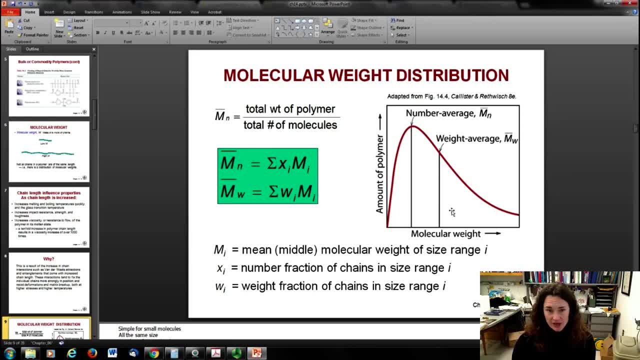 little bit to the higher molecular weight side here to the right. so the way that you calculate these two different numbers is: the number of molecular weight is the total weight of the polymer, polymer divided by the total number of molecules, And then the weight: average molecular weight. 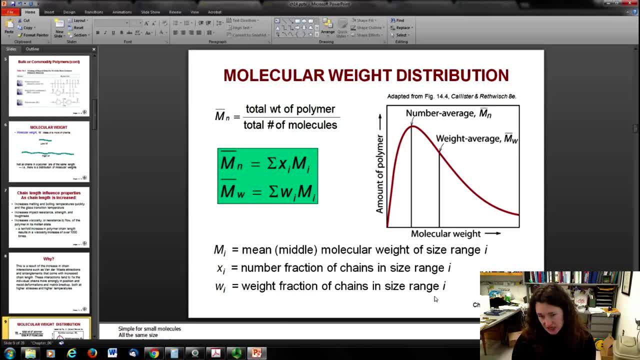 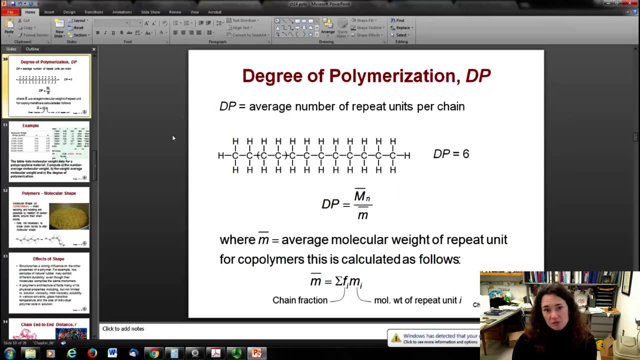 what you do to calculate that one is you multiply the weight fraction of the chain, times that value in the distribution. I'm going to do an example problem in a minute that I think will really clarify how these two numbers are calculated. Another important parameter is the degree of polymerization. The degree of polymerization is the average number of. 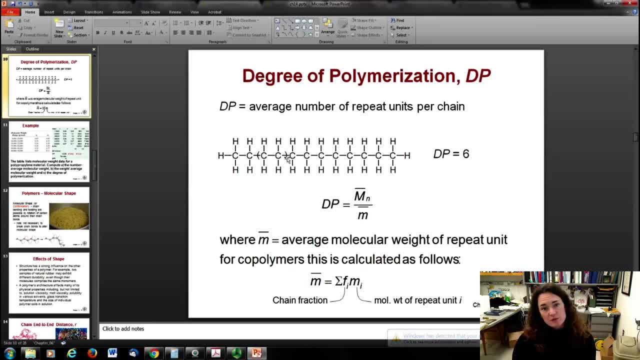 repeat units in a chain. So here, for example, if the repeat unit is these two carbon atoms, then you can count it up: One, two, three, four, five, six, And so the degree of polymerization here is six. You can calculate numerically the degree of polymerization by taking the. 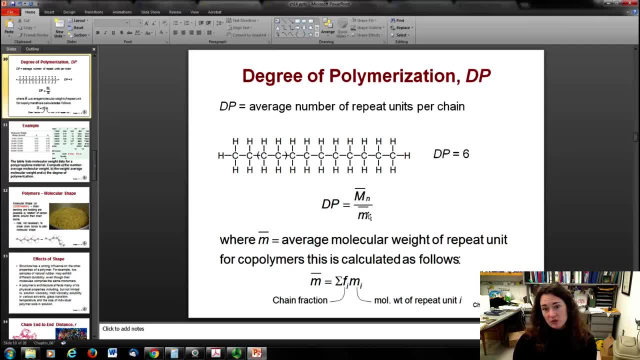 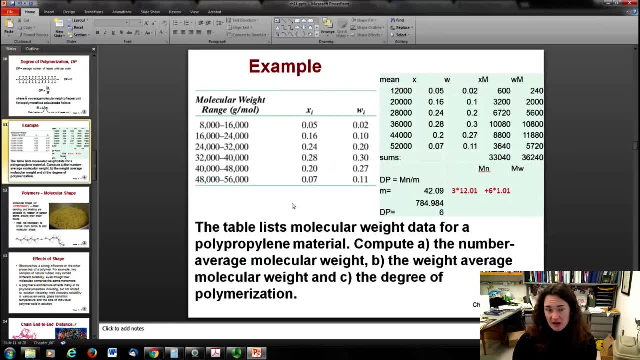 number, average molecular weight and dividing it by molecular weight of your repeat unit or monomer. So here's that example problem that I promised. So in this example problem there's a table, And this table lists the molecular weight data for polypropylene material. 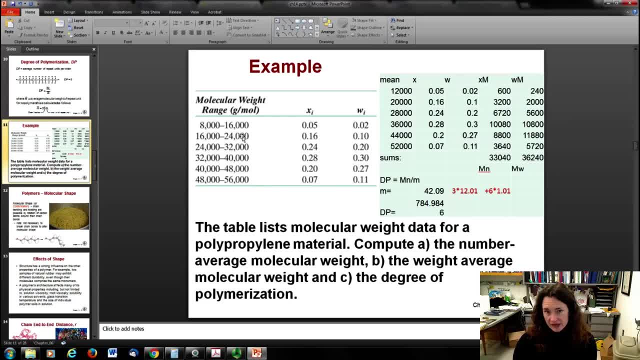 And so from this table, it gives you the molecular weight range in grams per mole of your molecules, And then it also gives the number fraction and the weight fraction. The number fraction is this xi and the weight fraction is the wi value. And then from that and this table, 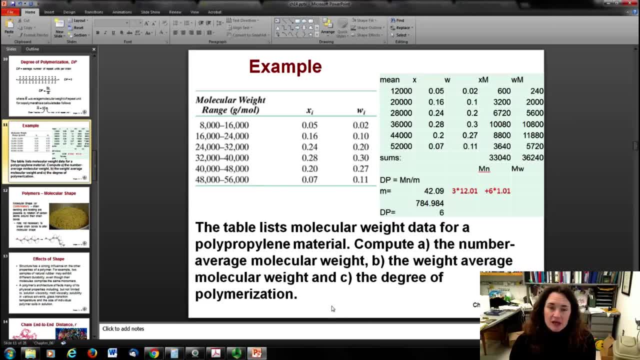 you can calculate the number average molecular weight And so what you can think of. if you go back to the distribution table, you can see that the number average molecular weight is on the right of your store 선 score. This is need to calculate the data in unit. 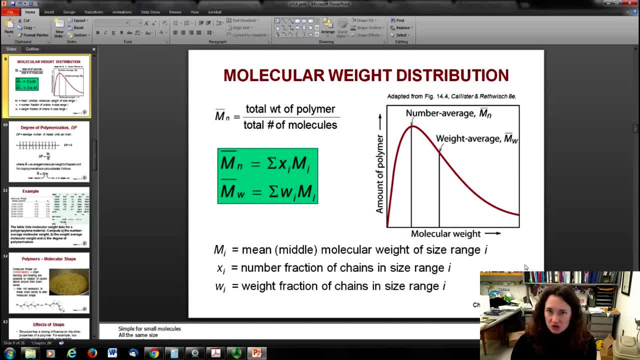 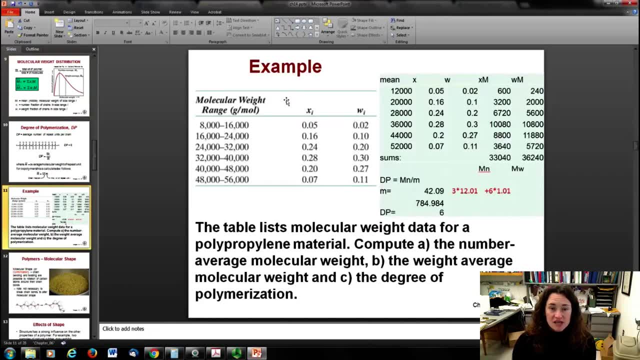 and电渦 value, which needs to be able to calculate the number average molecular weight power ratio. It reads 0,1 and then at the end you can find out where the correct Mazdel value equals an PCs dice between pi and pi maln. At first you need to calculate the formula for going from pi divided by piCause you're actually getting two values here. Now you can think of this as, instead of a continuous distribution function, maybe in terms of a histogram. okay, so you have a histogram or a bar graph of what these look like. Now, here the bars have widths given here, and the table and then the height of the bar graph would be given this way, And this is, if you're plotting it versus the number fraction or versus the weight fraction, okay, It would give you the height of that bar in two different ways. So, if it's 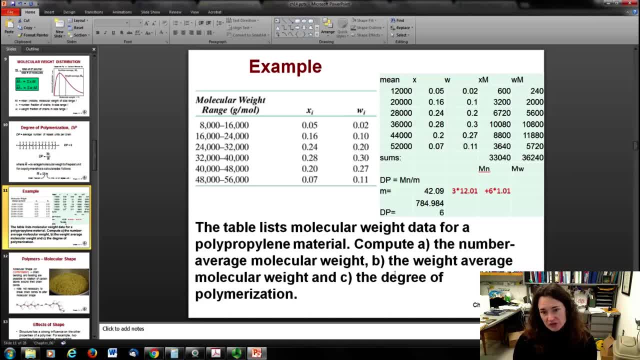 Okay, so to calculate the number, average molecular weight, what I've done here- here it is in the table, So I have a mean value. and what I did for my mean value was I just took the middle of this range and plotted it or put it in the table for each value. 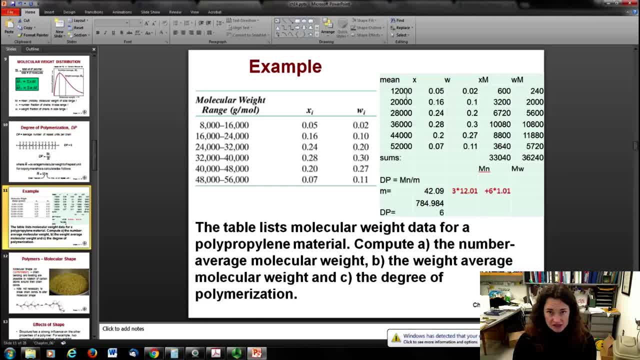 So, going between 8,000 and 16,000, I chose 12,000.. It was dead center in the middle. okay, So that's what I've done for each one of those values from that table and put it here. 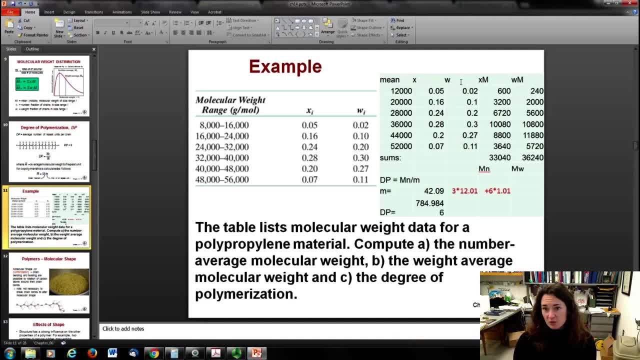 Now here is: I've copied and pasted over the number fraction and the weight fraction for each one of these two. just copied and pasted it directly and then I used that to calculate my number average and my weight average molecular weight. So this first column. here I take my values for the mean in column one and multiply it. 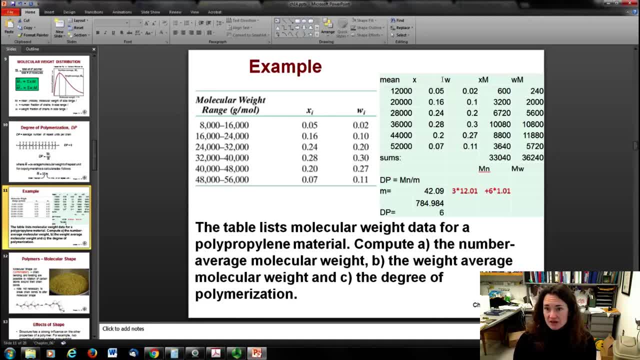 by the number fraction x here in column two and that I used for column four For my weight fraction. what I've done is I've taken my column one values and multiplied it by the weight fraction here in column two. That gives me column three and that gives me column five. 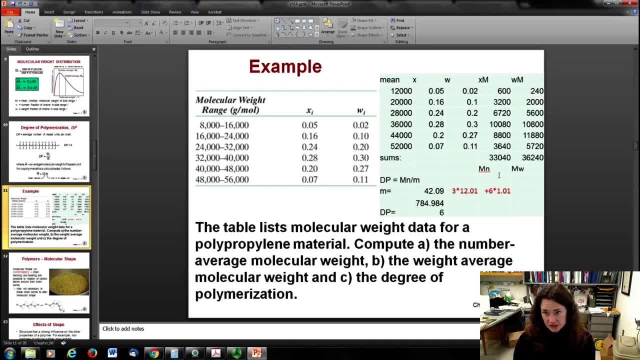 Now to compute my total number average molecular weight, what I do is I sum up all my column one values. So basically I've multiplied every fraction times its mean value right there for each value and then I summed it all up and that gives me my number average molecular weight. 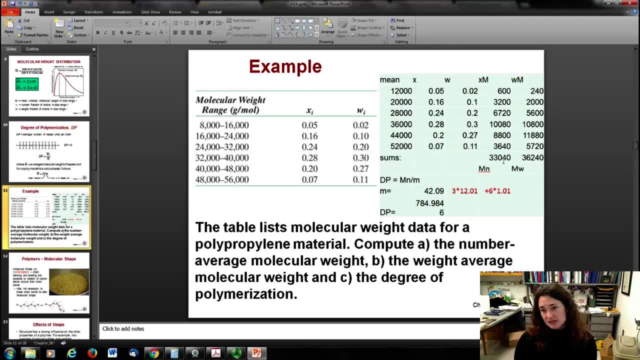 So my number average molecular weight for this is 33,040,. okay, because I summed up all the values here in this column to give me 33,040 for my number average molecular weight. So I'm going to take my number average molecular weight. 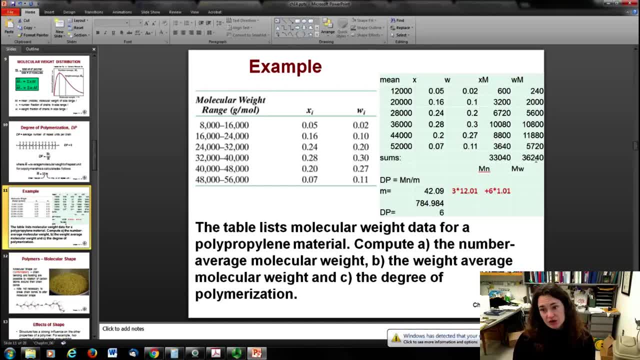 For my weight average molecular weight, I get 36,240.. Again, it's pulled to the right a little bit, as you would expect from the earlier plot that I showed you and that I got just from summing up all the values in column five here. 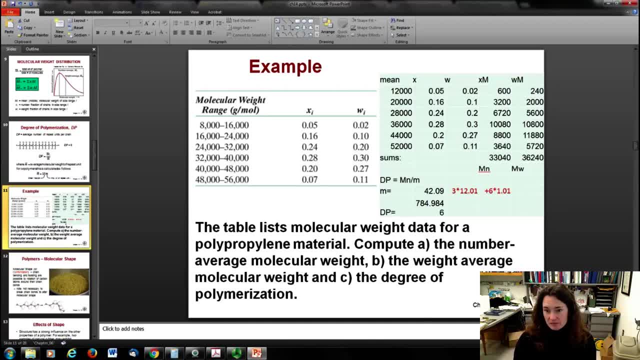 Okay, so there's my number average molecular weight, part A. my weight average molecular weight, part B. and for part C, I wanted to calculate the degree of polymerization. So the degree of polymerization, you take your number, average molecular weight, which? 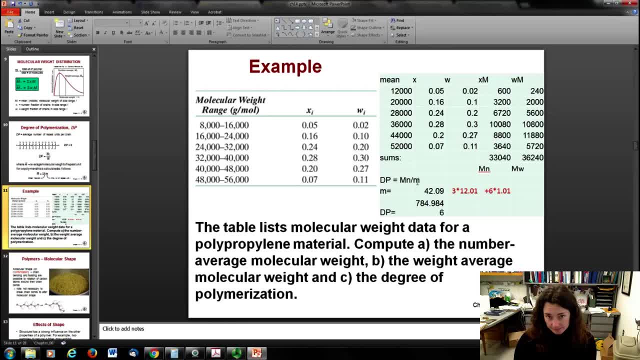 is your molecular weight and you divide it by the molecular weight of your repeat unit. okay, So the molecular weight of my repeat unit is 42.09 grams per mole. How do I know that? Well, it's polypropylene, okay. 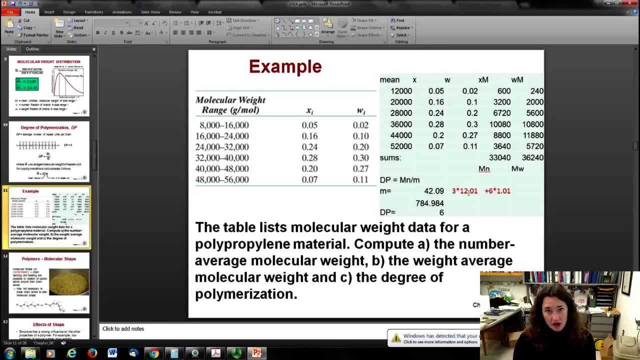 So propylene has three carbons. It starts out as propane, so it has- I'm sorry- propylene, so it has three carbons. Each carbon atom is 12.01 grams per mole, so I do three times 12.01, and then it's got. 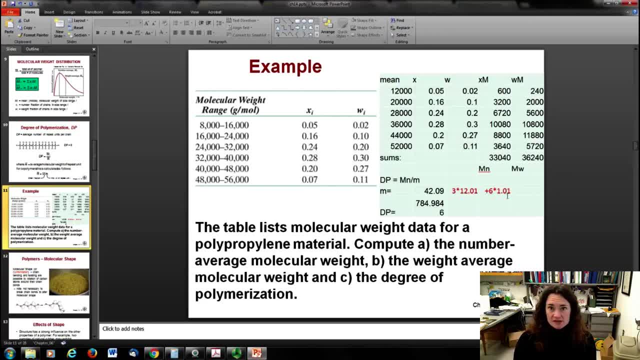 six hydrogen atoms. So each hydrogen atom has a molecular weight of, or an atomic weight of, 1.01 grams per mole. So it's three times 12 plus six times one to give me my value for my monomer, which is 42.09.. 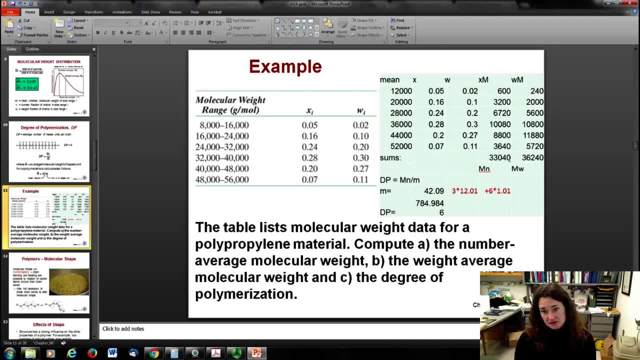 And then I take my number molecular weight, which is 33,040, and divide it by a 42.09, and that gives me my degree of polymerization, And so I get a lot of decimals here, but basically it would round to 785.. 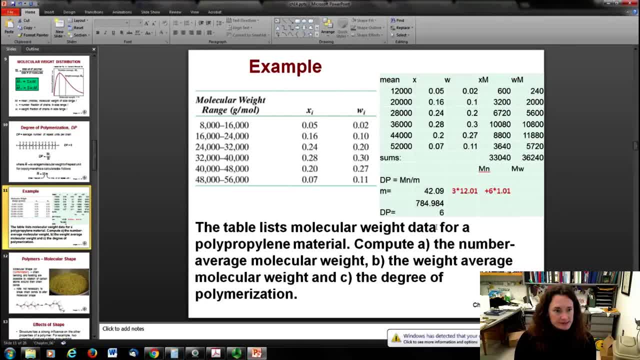 So that's a lot of decimals, I know. So in this case I've got a lot of decimals, I have a lot of coating on the material and I'm going to look at this and see if I can get around to it. 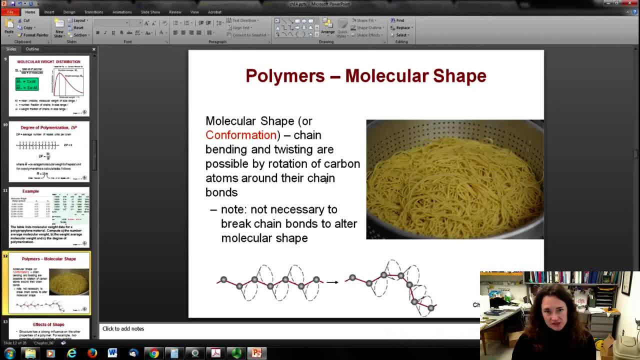 So I've got a lot of coating on the material. but in this case, what I can do is I can see that when I take my formula, what I can see is that my molecule has a hyperbolic shape. So I want to make sure that the molecule has a hyperbolic shape. 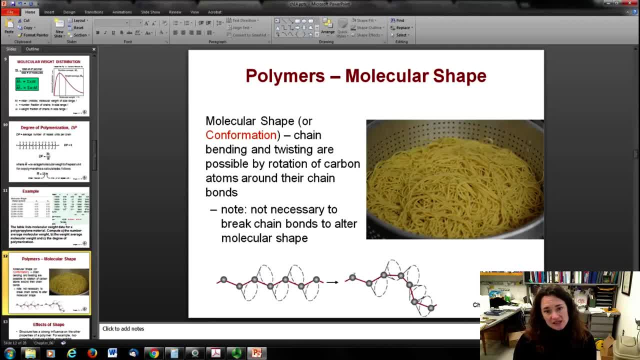 I'm going to take a molecule that's as big as a 13.5 particle and I'm going to take to alter the molecular shape. The rotation can just happen naturally, And what this allows the thing to do is to entangle with neighboring molecules, kind of like this spaghetti. So the 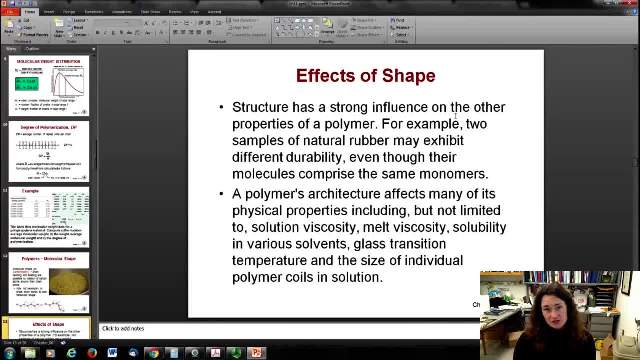 structure has a really strong influence on other properties of the polymer. So, for example, two samples of natural rubber may exhibit different durability even though their molecules comprise the same monomers. And a polymer's architecture affects many of its physical properties, and this includes, but isn't limited to, the viscosity, which we already talked about, the resistance to flow. 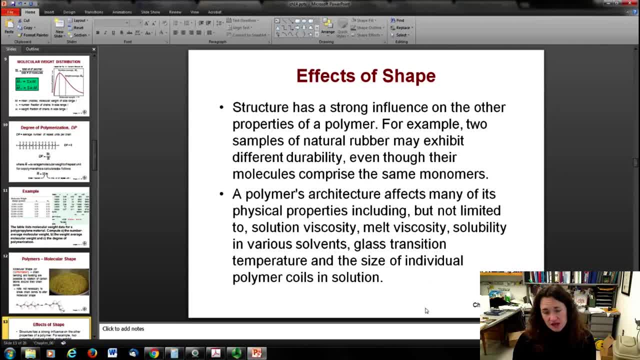 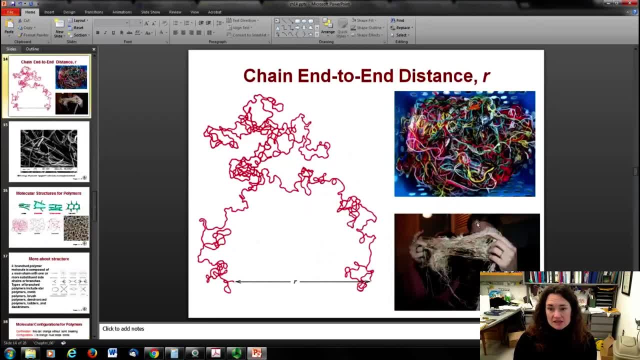 the solubility in different organic solvents, the glass transition temperature and the size of the individual polymer coils in the solution, And this can all be sort of put in terms of a parameter of the chain end-to-end distance r. This kind of gives you how much the polymer entangles. 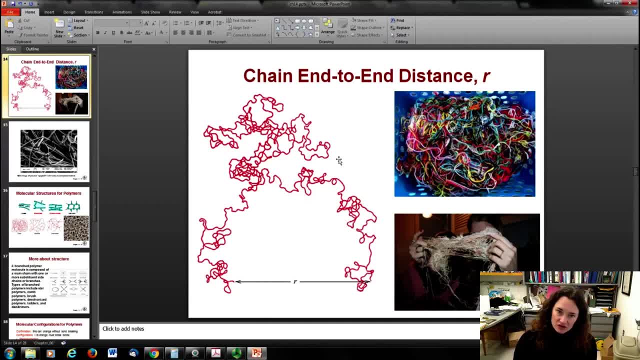 with itself in the neighboring molecules. So the more entangled it gets, the crazier it gets, the harder it is to entangle. So the more entangled it gets, the crazier it gets, the harder it gets to pull apart. the higher its resistance to flow and the less its solubility is in different 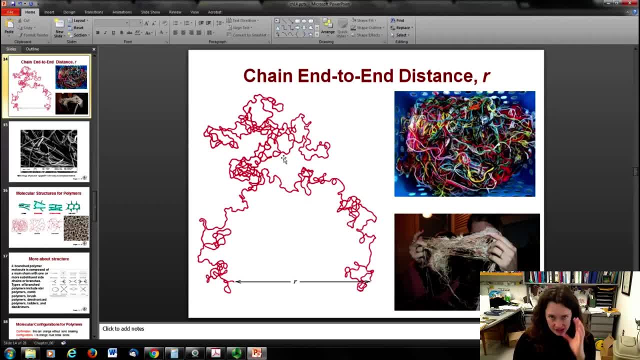 solvents, And that can be explained by thinking about how difficult it is just to entangle yarn or a necklace chain. It's nigh onto impossible sometimes, And so you can imagine that if it's on the molecular level and things are getting entangled, that really isn't going to change. 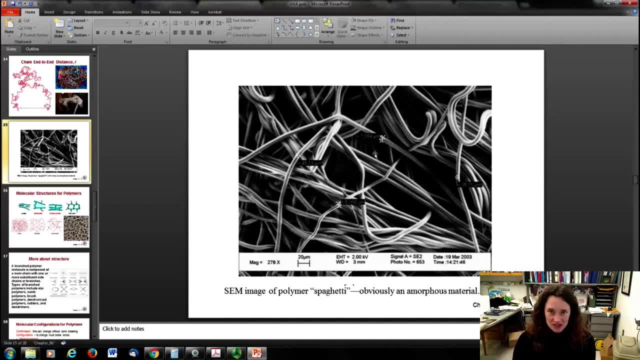 Here's an SEM image that I showed earlier in the lectures of polymer spaghetti, So you can see here it's on the nanometer scale. It's getting entangled. I'm sorry, the micrometer scale is getting entangled. It's crazy. It's not going to be any different when you shrink it down even further. So there's. 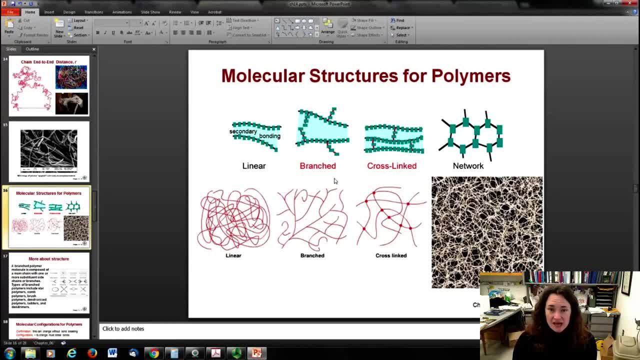 different kinds of molecular structures that polymers can have, And these molecular structures can also impact the polymer's performance. So, for example, you can have a linear polymer like polyethylene, I'm sorry, And that can have a certain kind of structure. You can have a branched polymer, And if you have a branched polymer, this is similar. 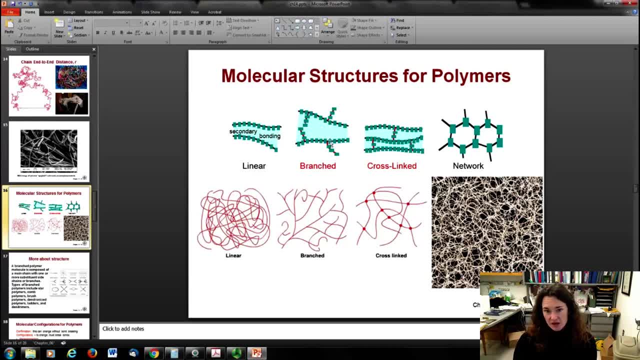 to polymethylmethacrylate perhaps. then you have these side chains that come off, So that's your branched polymer. You can have cross-linked polymers, And that's when the polymer chains actually form bonds with neighboring chains, So you'd have a bond sticking between the two. 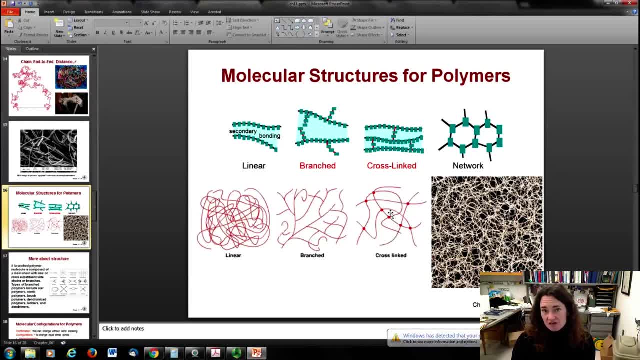 polymers like that. Cross-linked polymers are stronger and tougher than other polymers. For example, your car tires are heavily cross-linked And then you can have work polymers where the polymers are bonding like crazy with any polymer that crosses its. 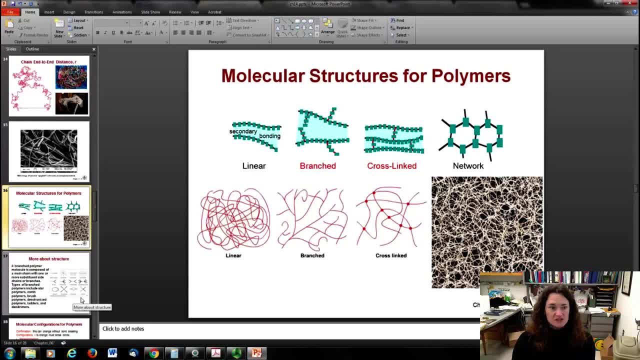 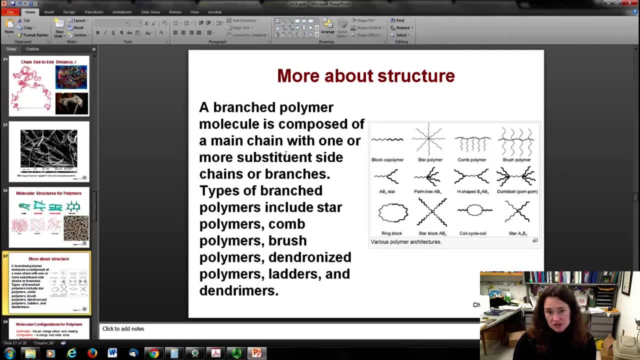 path And these are very, very tough and resistant to wear. Branched polymers: we talked about these, But branched polymers can have a main chain with one or more substituent side chains or branches, And then they can have all kinds. 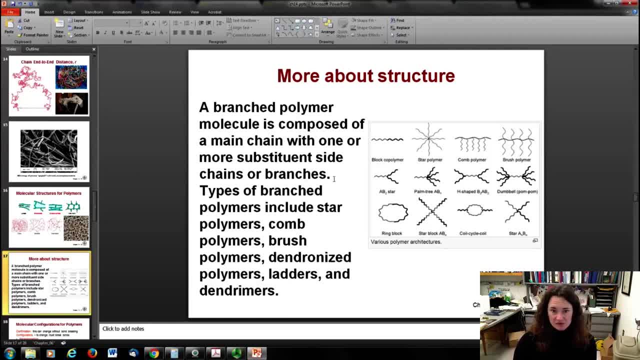 of really, really fun, interesting shapes that lead to different properties. So some examples of this types of branched polymers: star polymers coming off like that make little stars. Comb polymers looking like a comb. Brush polymers coming off either side Dendronized. 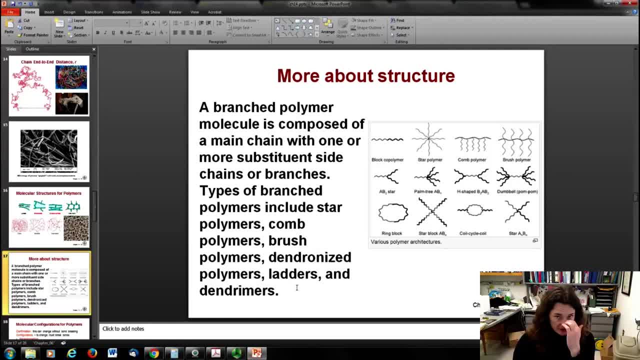 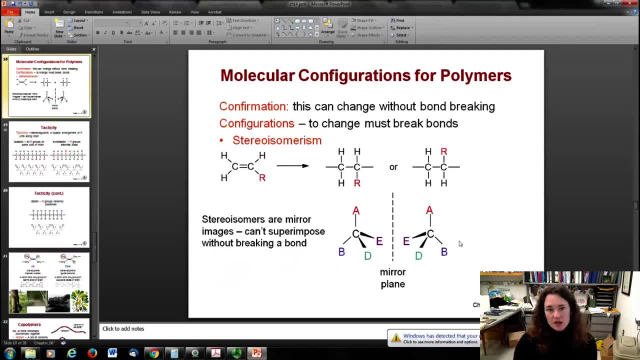 polymers, ladders, dendromers, they all form these different structures And because they have these different physical structures, they have different properties. Now, configuration is different from conformation. They often get confused, but they are actually different. The conformation, as we discussed, can change without bond breaking. It can just. 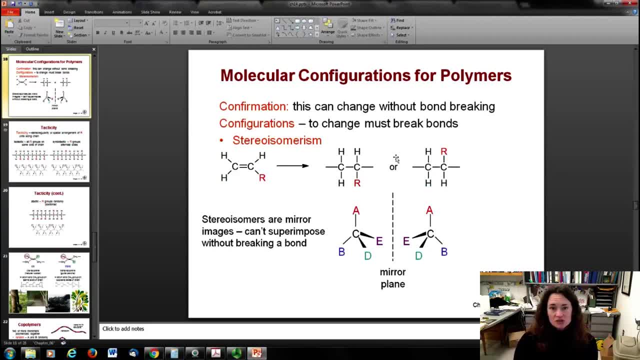 rotate within the bond. So in order to change the conformation, in order to change that, you do have to break the bond. So one example of that is the stereoisomer. So for example, this has the same chemical formula but the side group is on a different side. It's kind of a mirror image of itself. 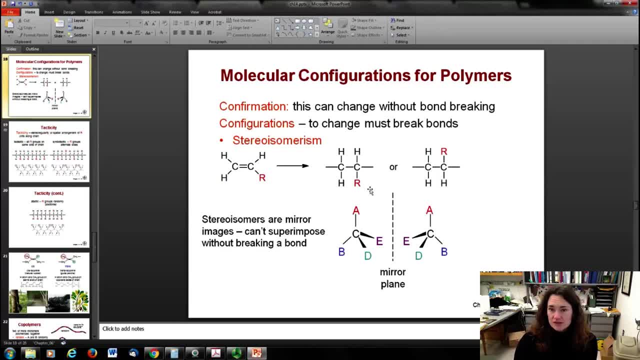 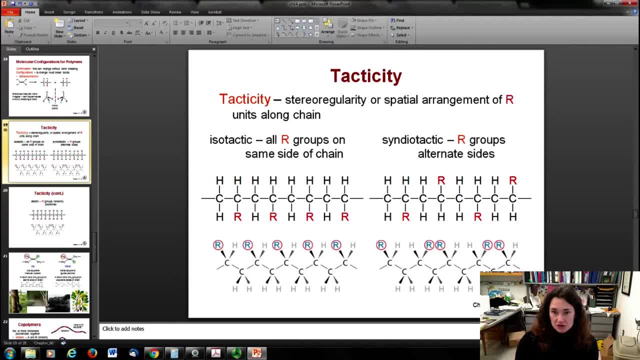 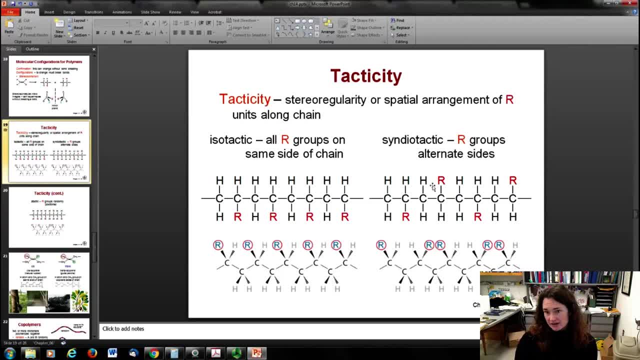 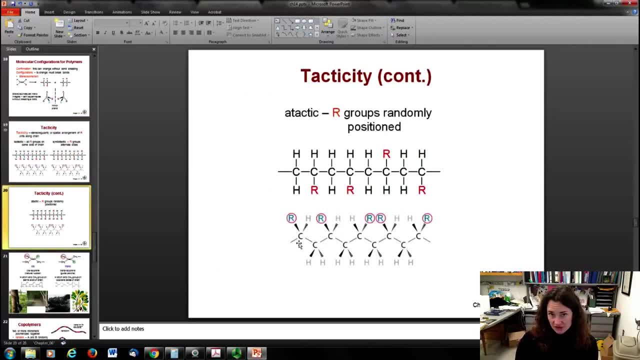 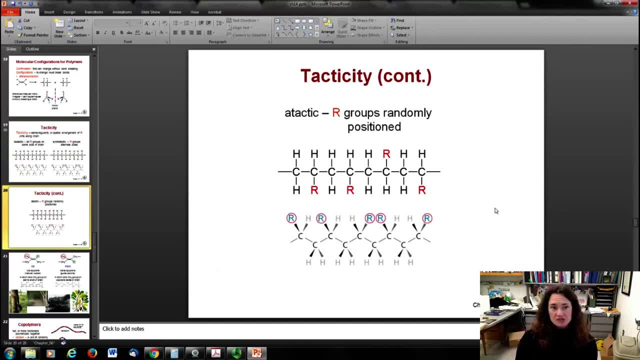 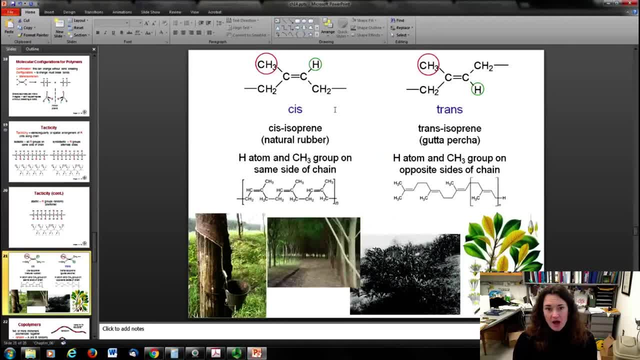 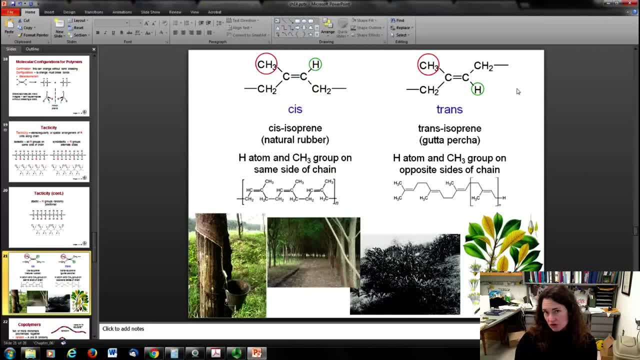 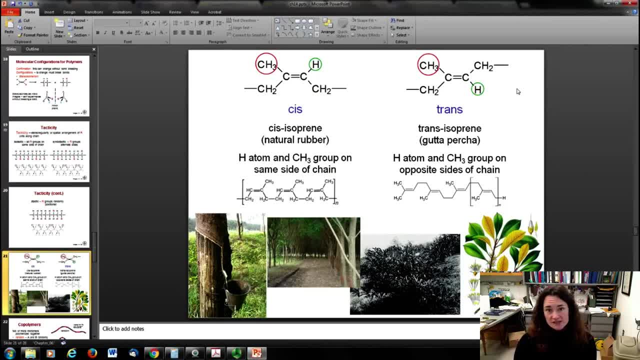 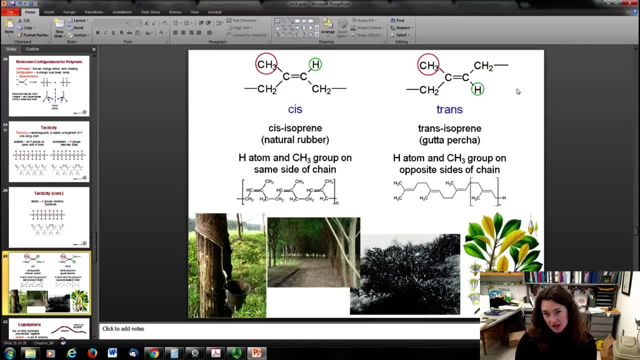 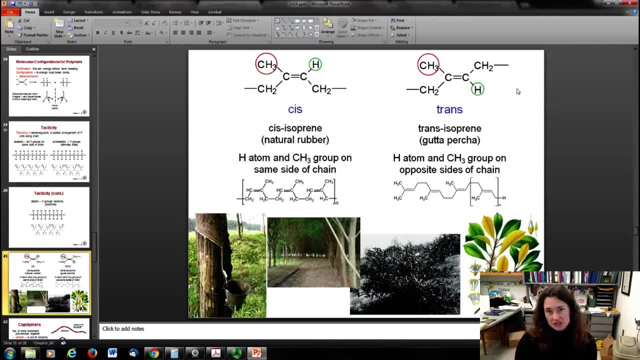 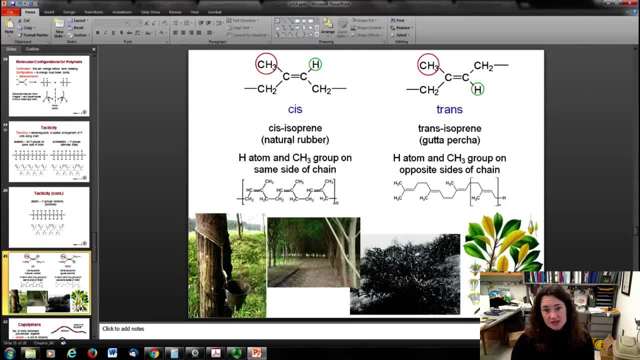 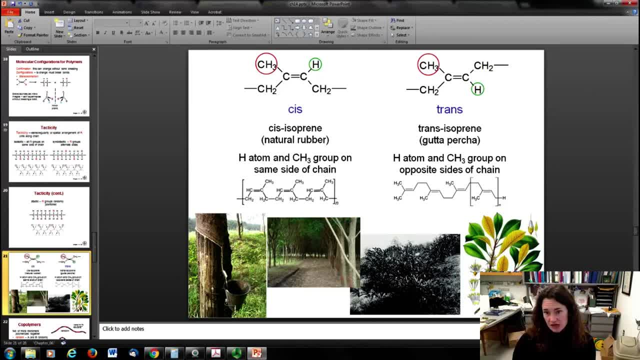 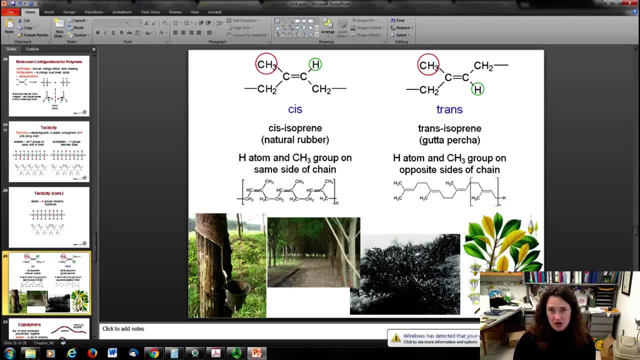 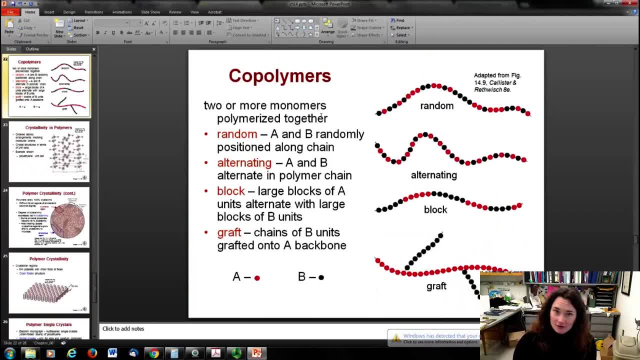 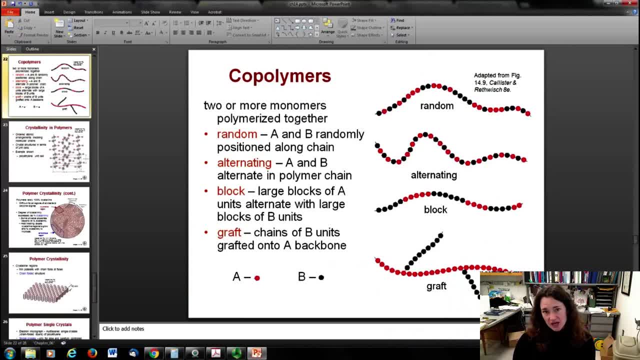 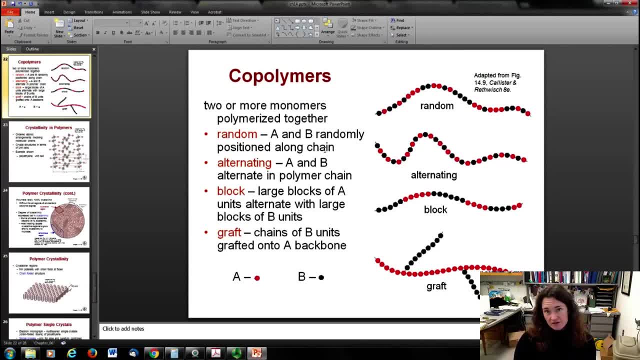 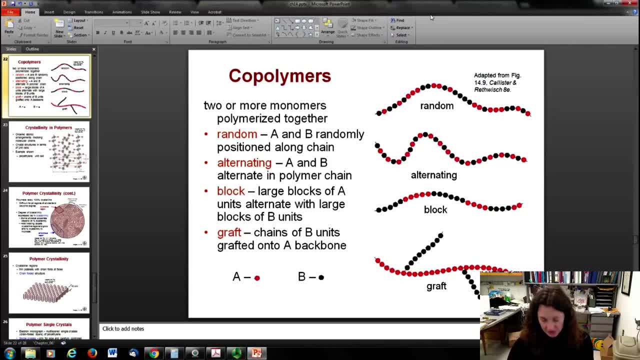 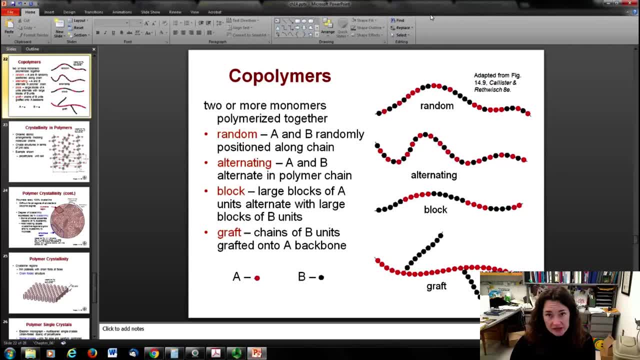 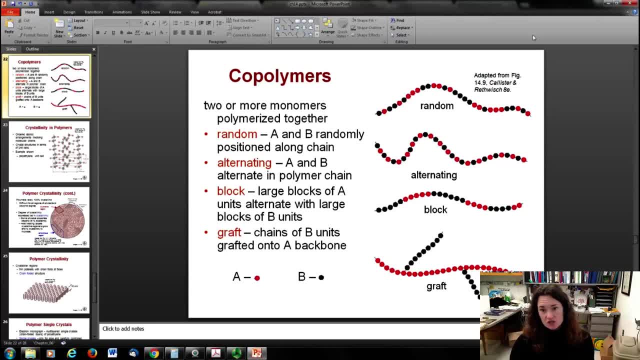 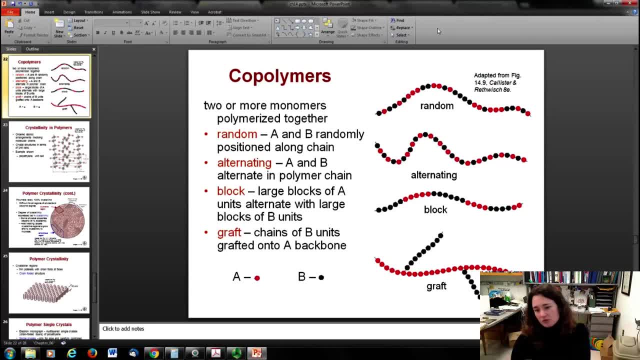 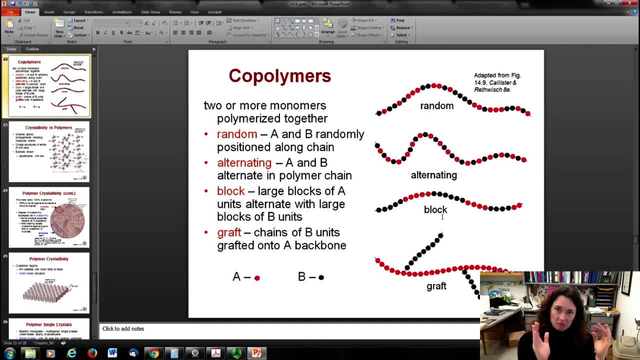 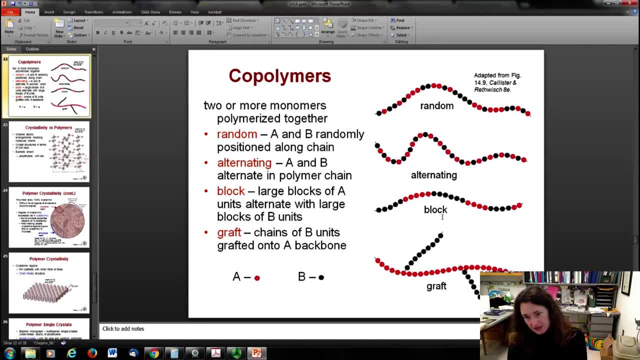 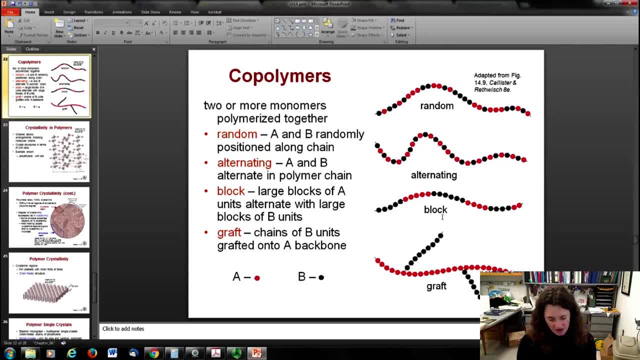 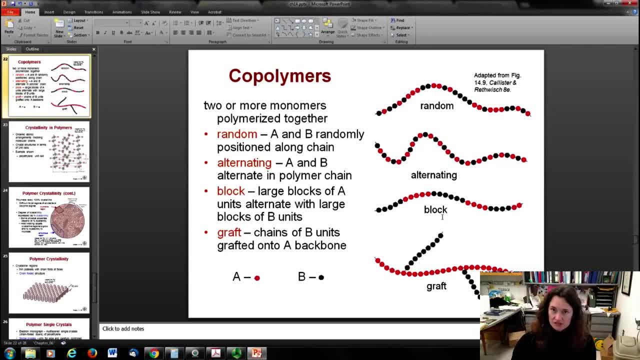 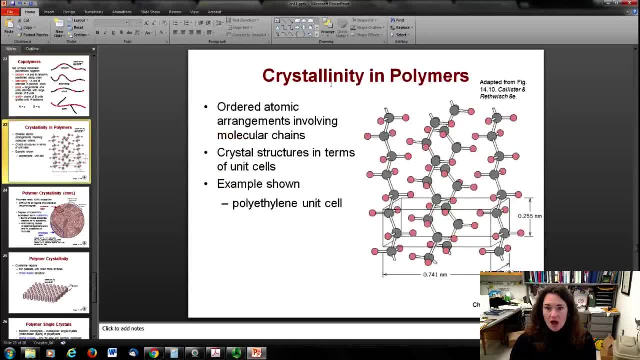 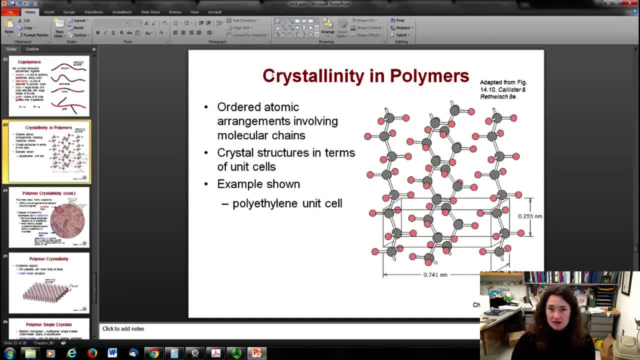 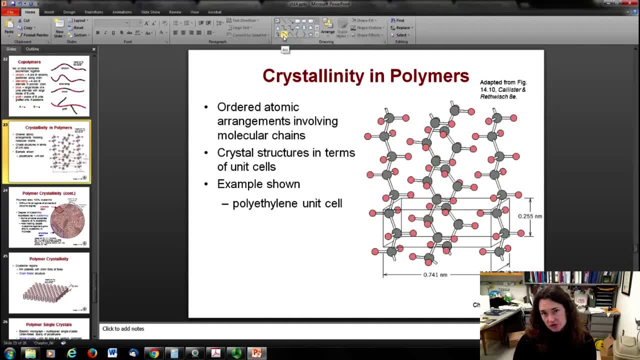 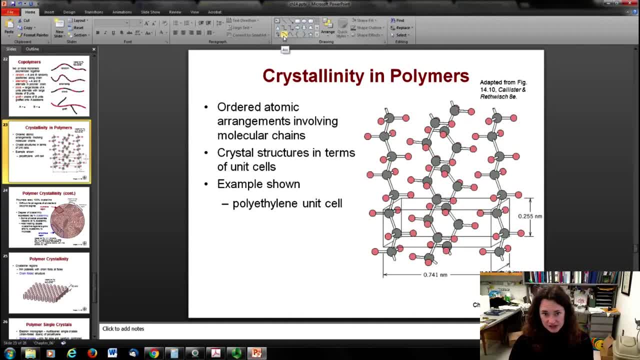 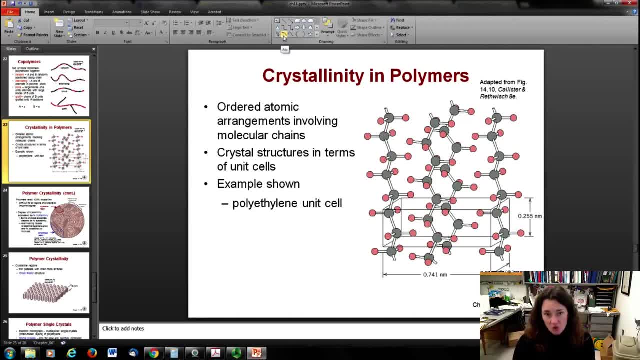 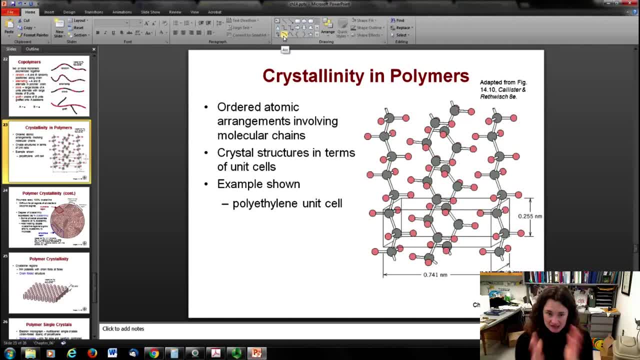 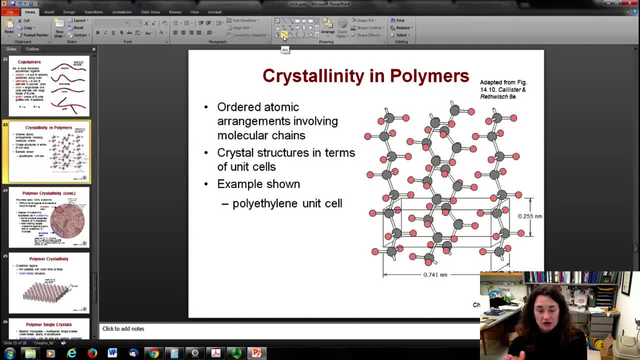 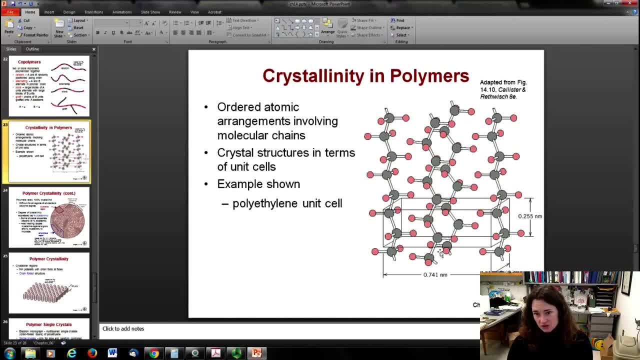 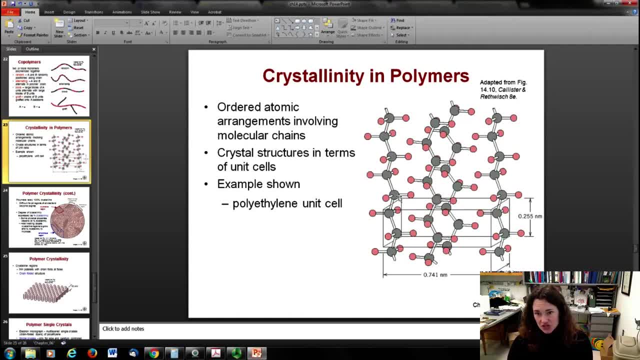 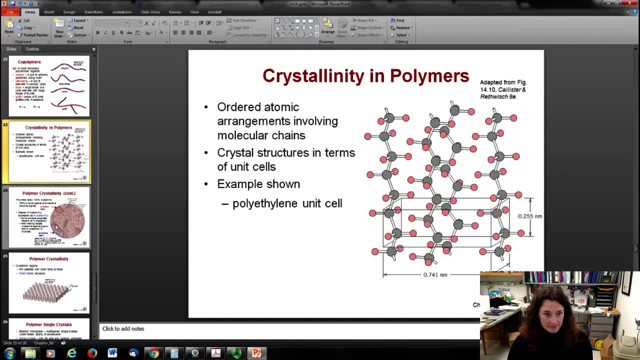 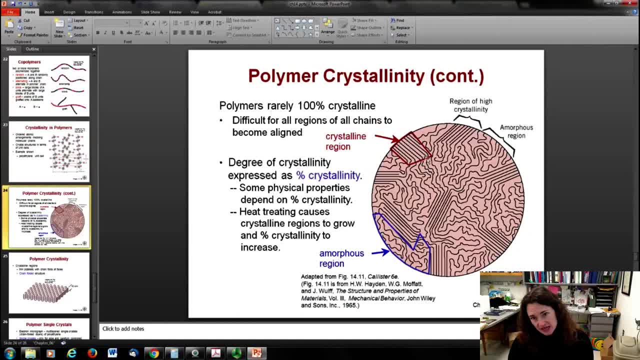 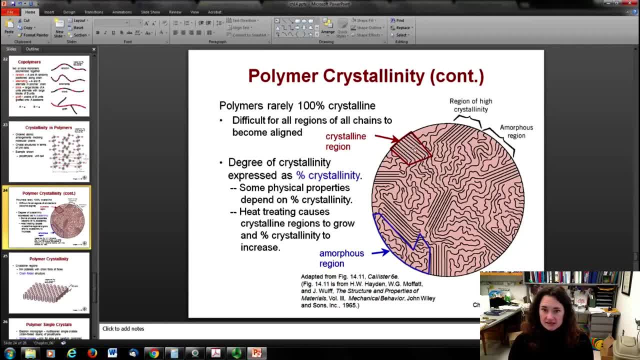 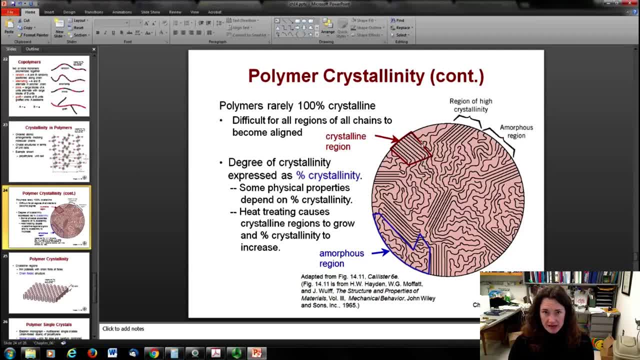 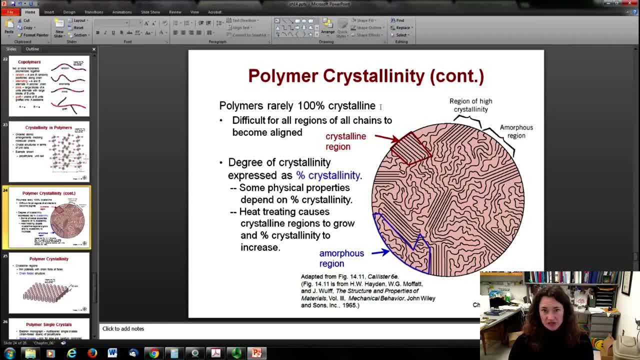 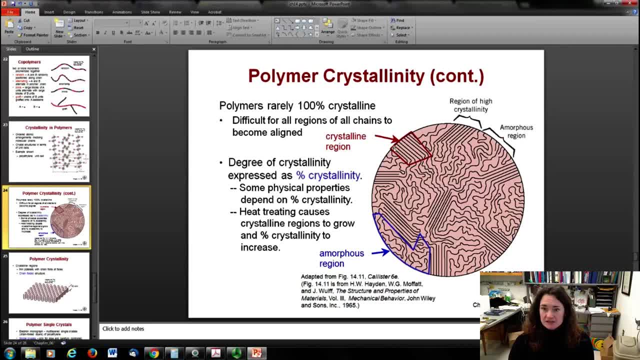 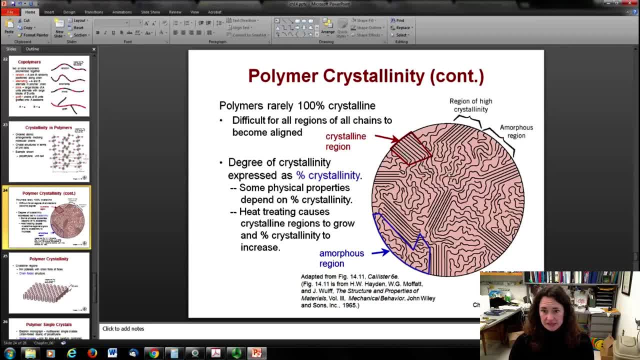 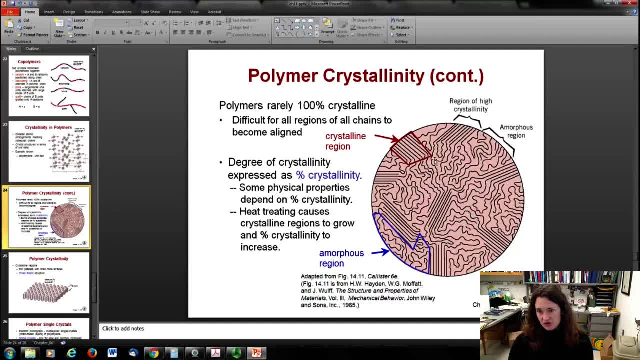 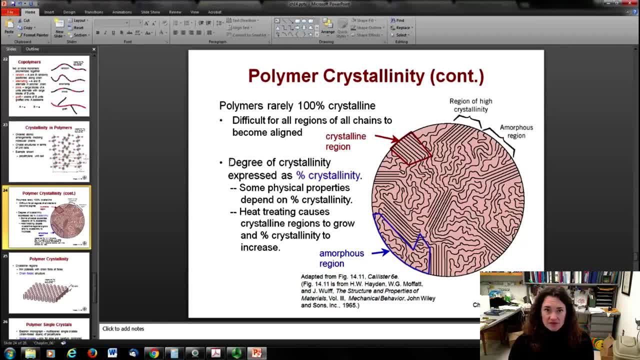 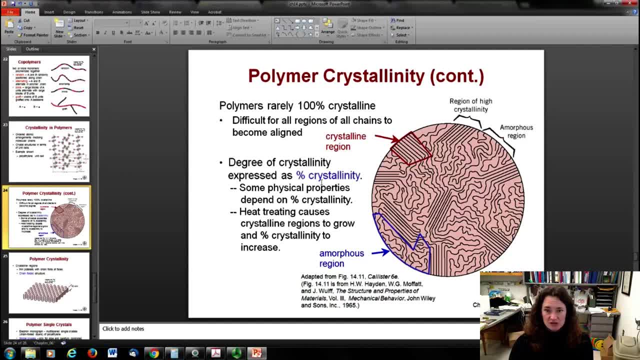 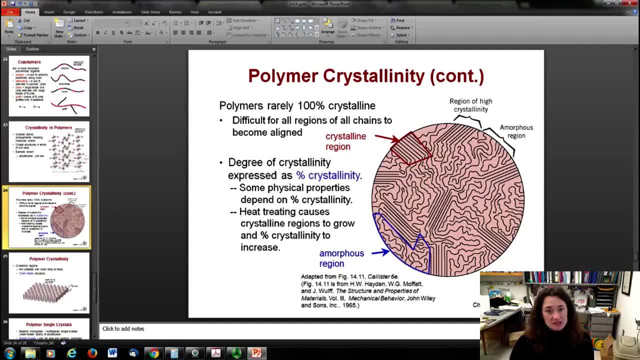 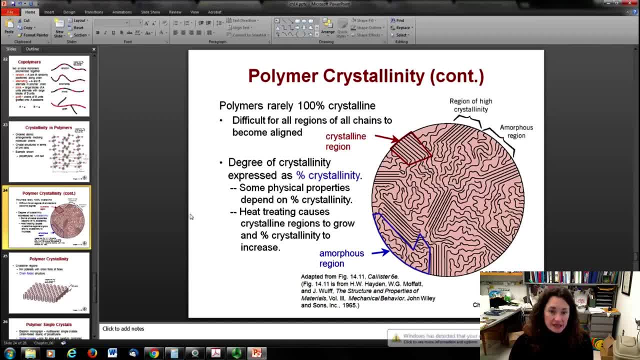 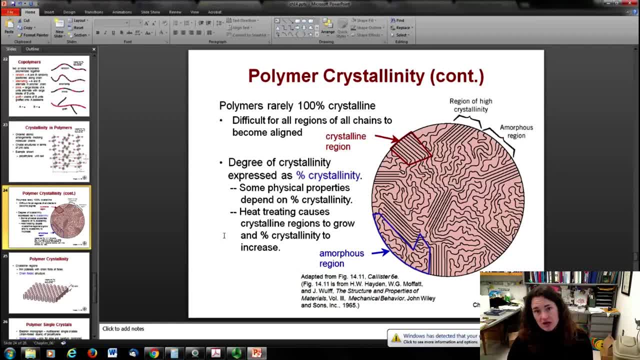 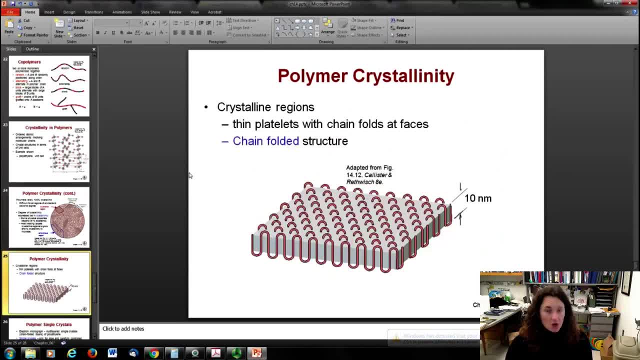 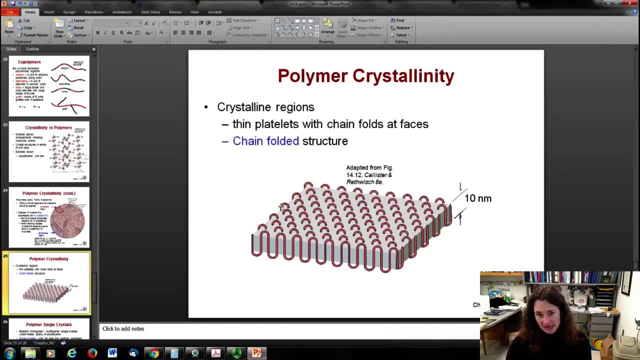 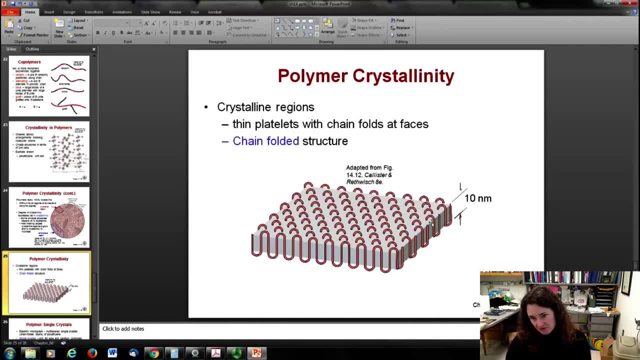 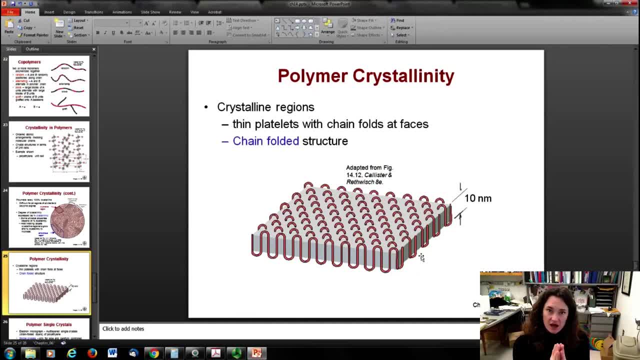 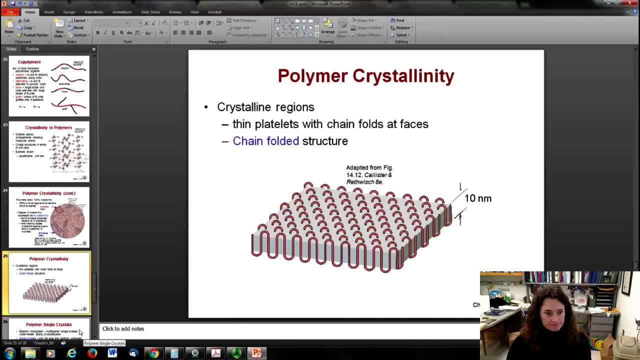 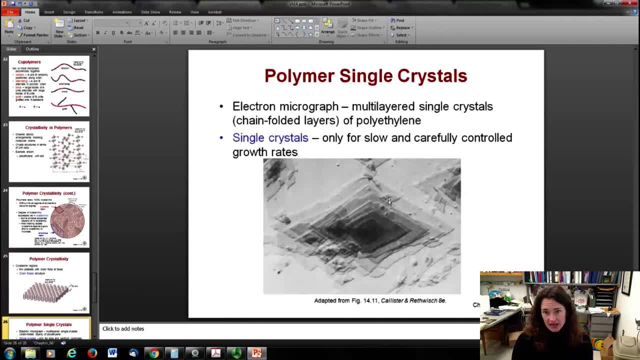 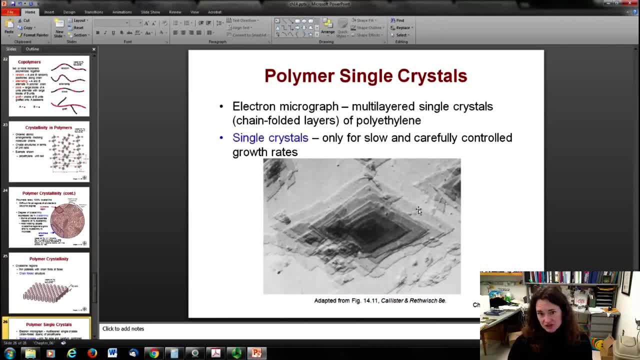 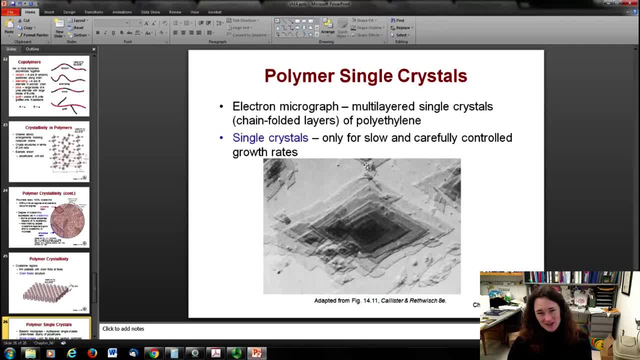 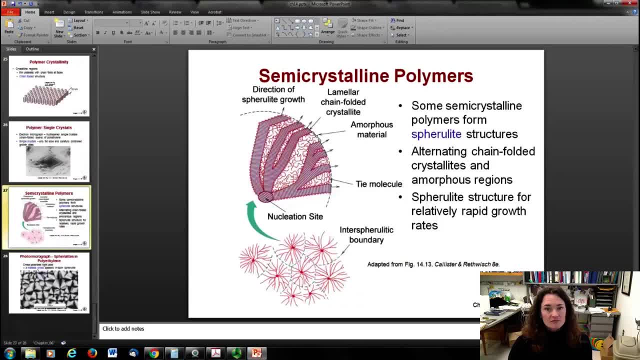 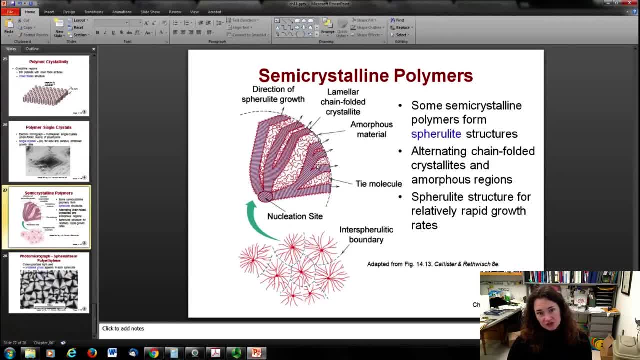 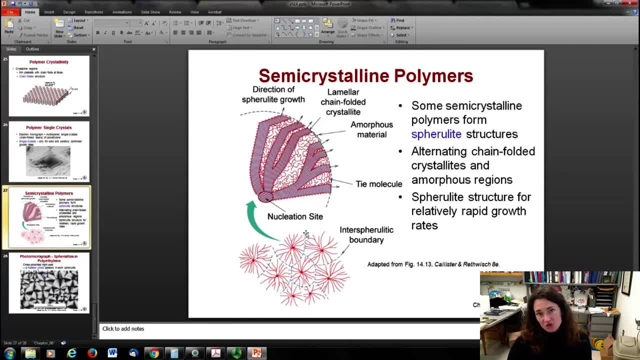 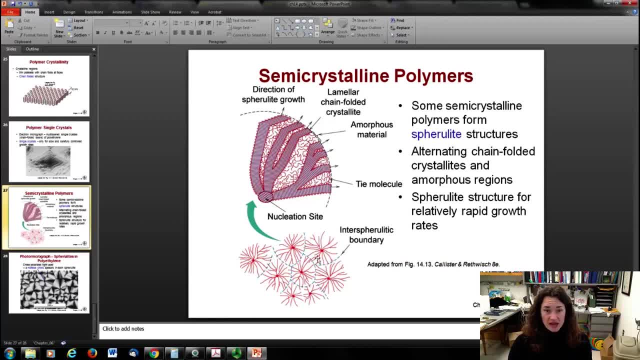 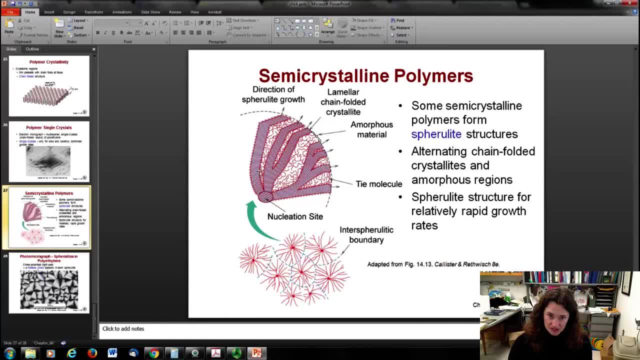 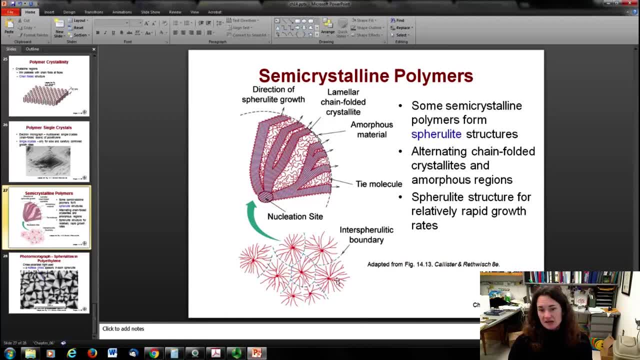 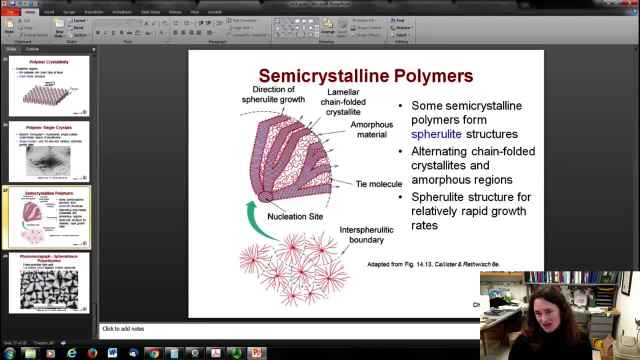 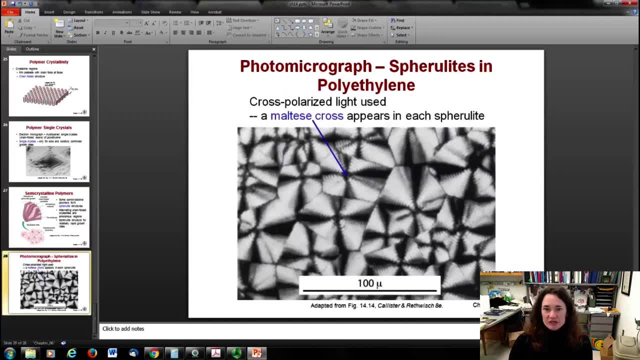 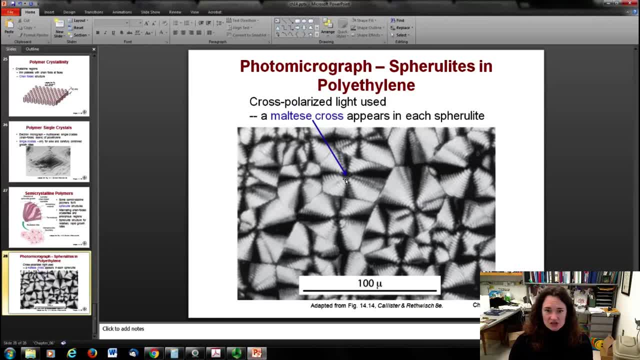 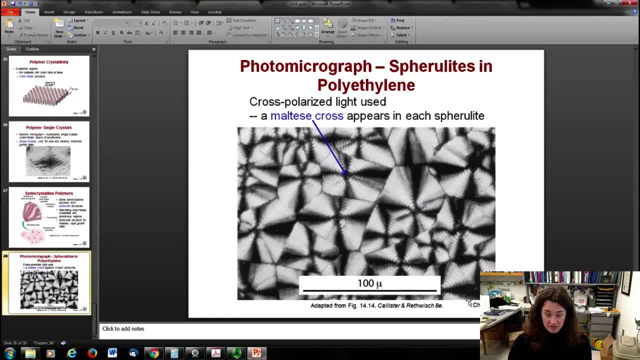 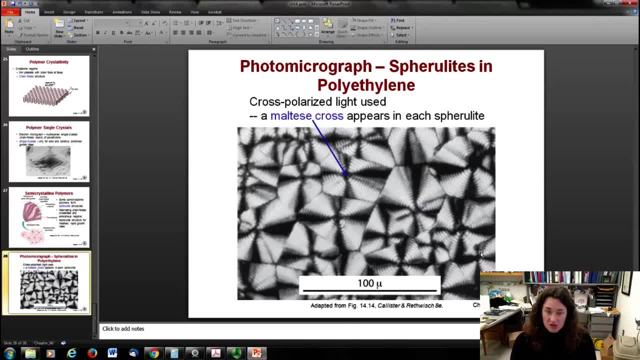 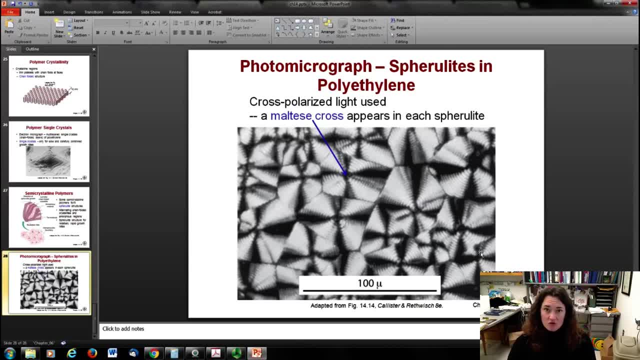